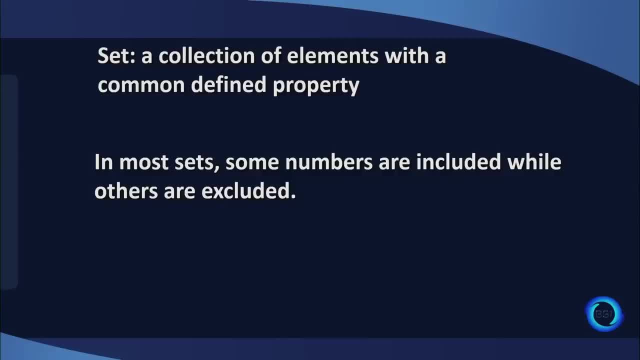 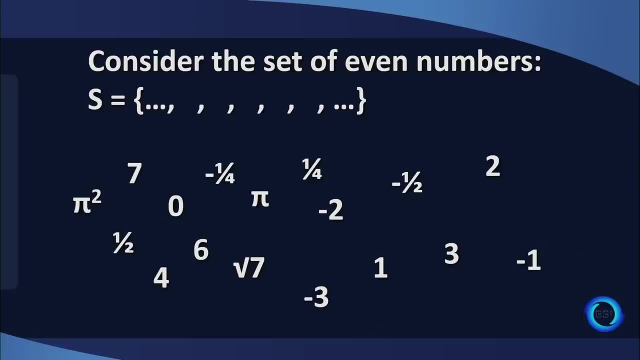 make up this set And what I think it is. it's a group, in this case, of numbers that have a common defined property, And so you can have different types of sets out there, And in most sets some numbers are included in the set and other numbers are excluded from the set, And it's 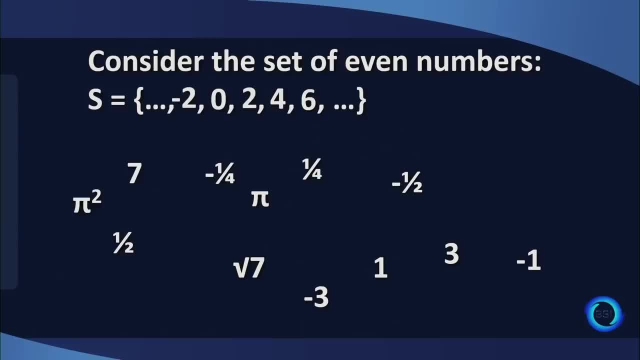 other numbers would be excluded from it. That's pretty easy. That's the set of even numbers. We could consider the set of negative numbers. Now, that's a different set, isn't it? And so a different set of numbers will be included in there, and then those other ones will be excluded. 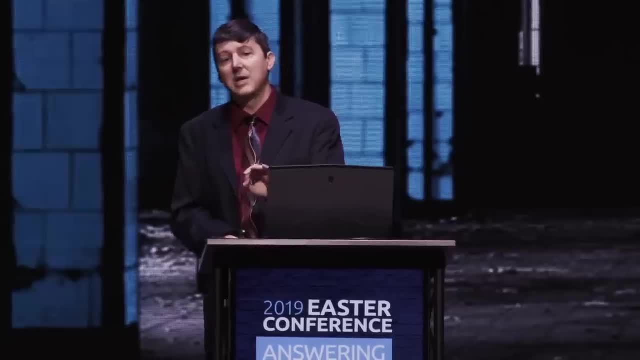 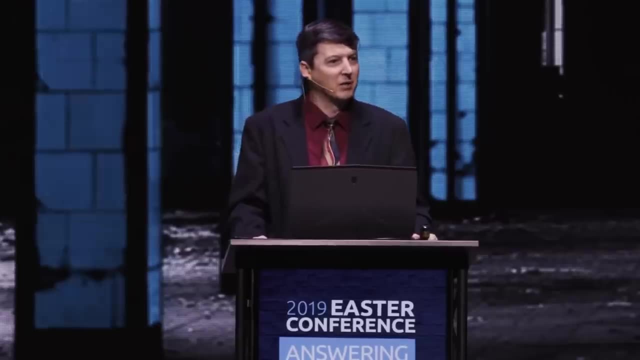 Now for those two sets. you can tell just by looking at the number whether or not it belongs. right, In this case, if it doesn't have a little negative sign in front of it, it doesn't belong, And if it does, it does belong. So that's pretty easy. You can tell just by looking at the number. 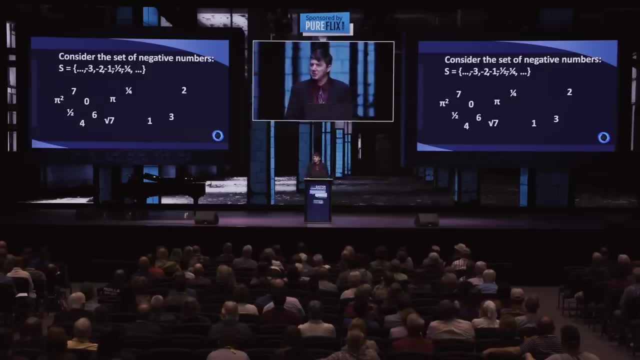 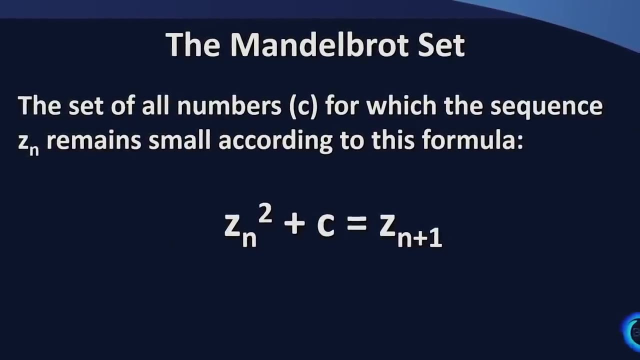 But there are some sets that have a more complicated definition and you can't tell just by looking at the number whether or not it belongs, And so we're going to talk about a particular set that's called the Mandelbrot set. This was discovered in the late 1970s, early 1980s, named after the person. 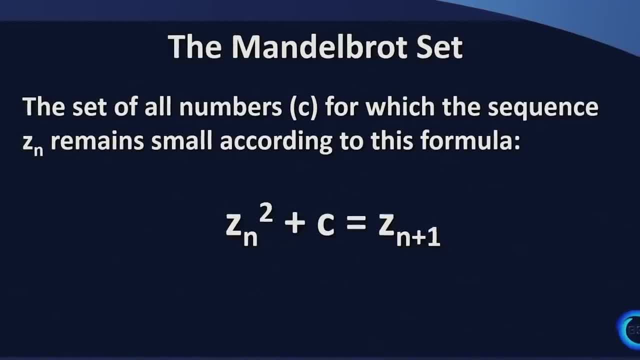 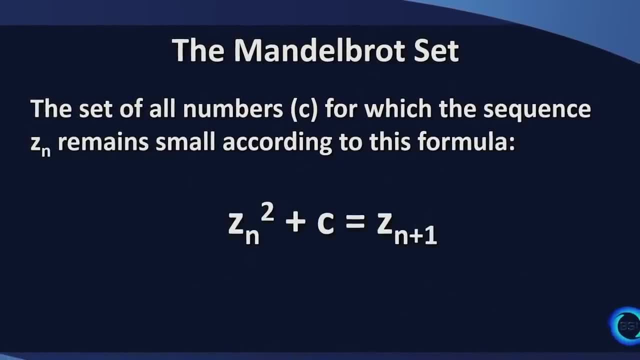 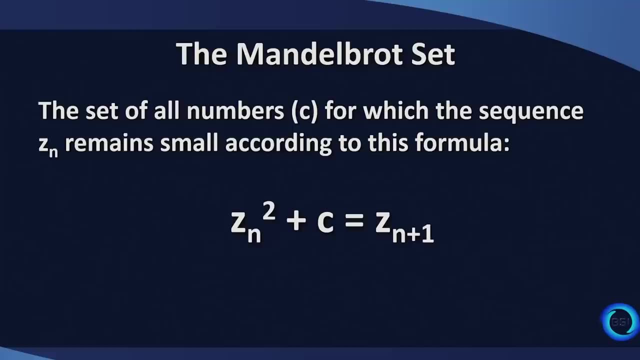 who really discovered this? Benoit Mandelbrot. He was a math guy and a computer guy. He worked at IBM. This set is defined according to this little formula that you see right here, where it's the set of all numbers: c. c is a number that is potentially part of the Mandelbrot. 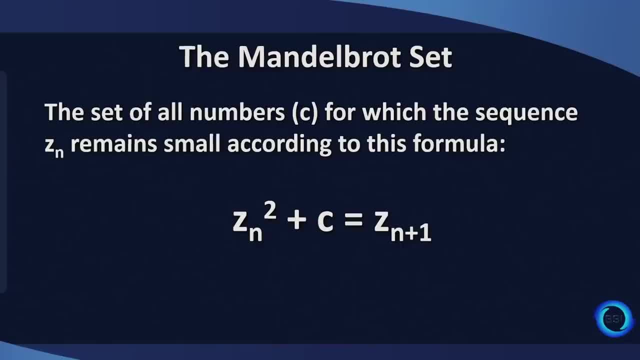 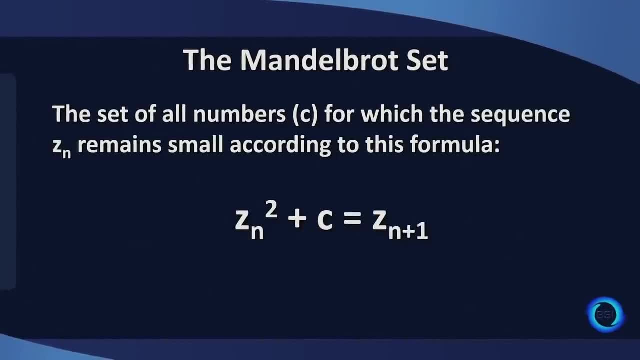 set- We're testing it- For which this other number, z, remains small. according to this little formula- And it looks very complicated, but it's really not, I'll take you through it- The little n just means that that's a particular value of z. n plus 1 is the next value of z, So there's lots of values. 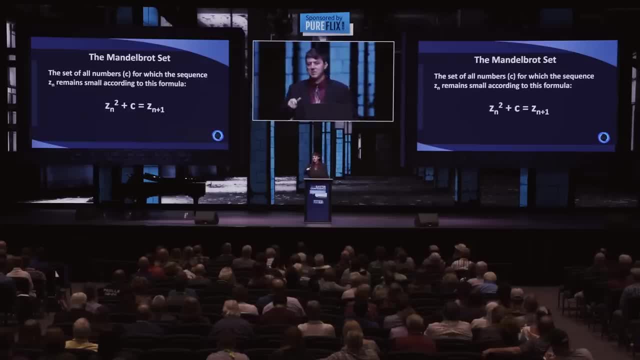 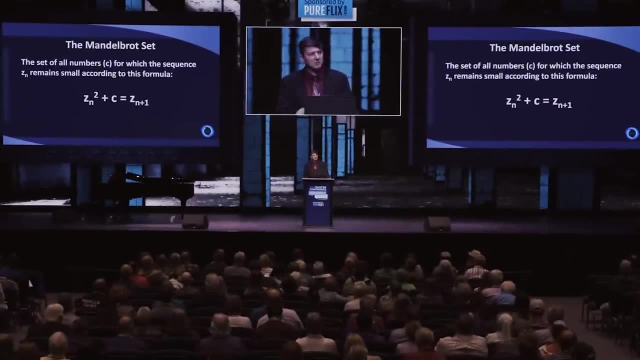 in the sequence And if that sequence of z stays small, then the other number, c, is part of the Mandelbrot set. On the other hand, if the sequence of z gets very big, if it goes 1,, 2,, 100,, a million, 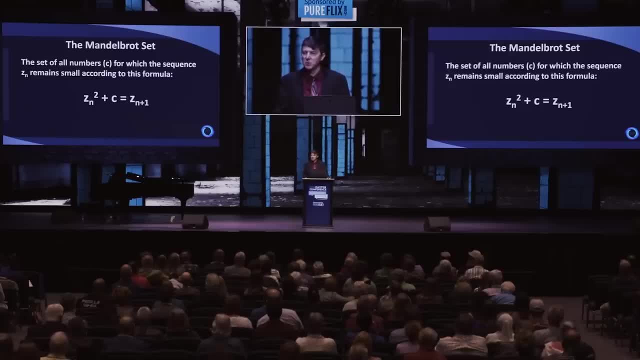 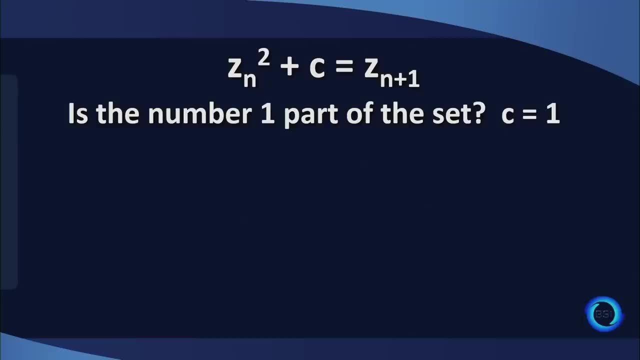 a billion, then c is not part of the Mandelbrot set And we'll do a couple of examples to let this sink in. It's pretty straightforward really. So we're going to ask: is the number 1 part of? 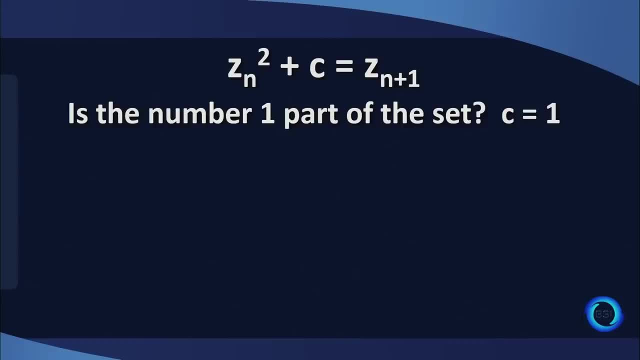 the Mandelbrot set. So c equals 1,. okay, And we're going to plug that into our formula then. So we have z squared plus 1, because that's the number we're testing. That becomes the new value of z. Now the first value. 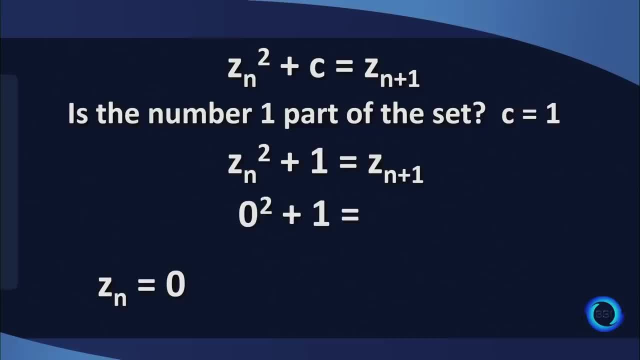 of z is 0 by definition, So that's the first value. So we plug that in and we have 0 squared, which is 0, plus 1 is 1.. Yeah, 0 squared plus 1 is 1.. So that's the next value of z. okay, And 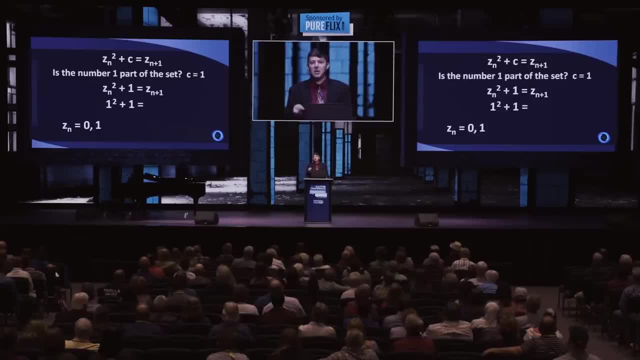 what we'll do is we'll put that 1 back into the formula. That's the new value of z. So now we plug that back in. So we have 2 squared is 4.. 2 times 2 is 4, plus 1 is 5.. Okay, you're getting. 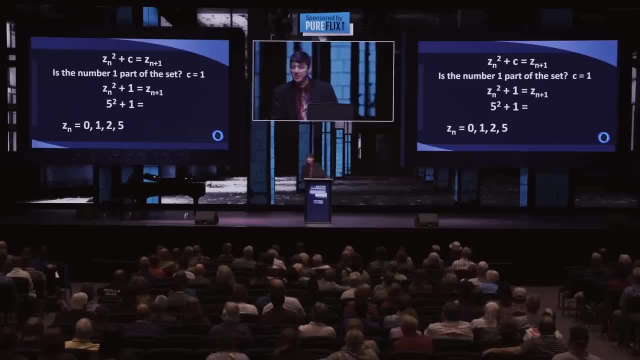 this: You put it back in: 5 squared 25, plus 1 is 26.. Okay, we put that back in. 26 squared is a big number and you put that back in. Okay, now you see what's happening here. 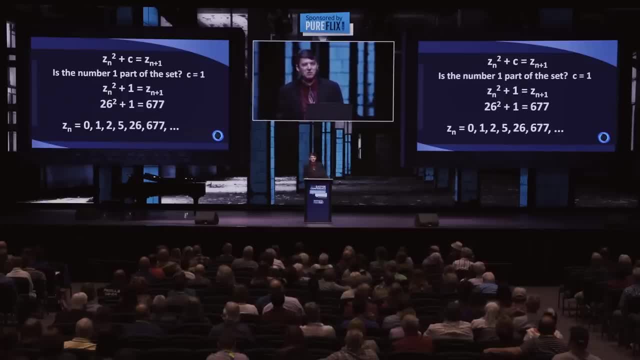 Is the sequence of z staying small? No, So is the number 1 part of the Mandelbrot set? No, because it has to stay small for it to belong. There's one more complication and then we get to the really cool stuff. The other complication is that the Mandelbrot set 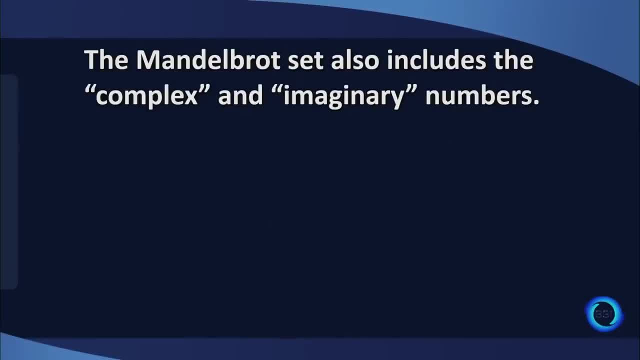 also includes what are called complex and imaginary numbers. okay, So an imaginary number is a number that when you square it, you get a negative number, and that's a little hard for us to understand, and so they call them imaginary. It's just a name. I hate that they have that name. 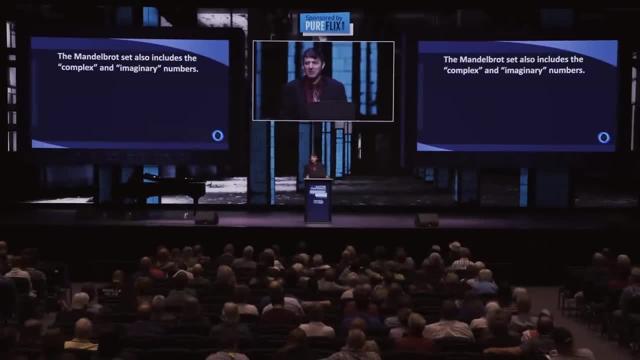 because it makes it sound like they don't exist. You know they're fabricated. No, they do exist. imaginary numbers do exist. and to add insult to injury, the numbers that are not imaginary they call real. but it's just, that's just terminology. Both are equally true. let's put 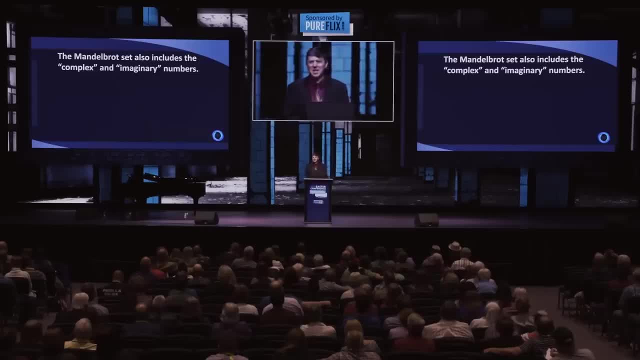 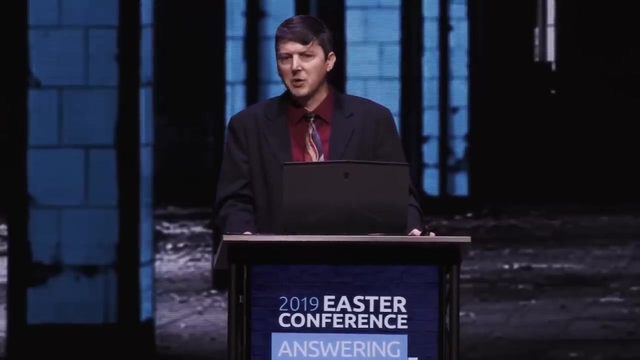 it that way. but how do we have a number that times itself as negative and it's represented by a lowercase i? That's the kind of the primary imaginary number when i times i is negative 1. How do we make sense of that? After all, imaginary numbers are not positive, because a positive number squared is positive, And yet the imaginary number times itself is negative. Imaginary numbers are not negative because a negative number squared is also positive, and imaginary numbers are not zero because zero squared is zero Weird. So we have a number that's not positive, it's not negative. 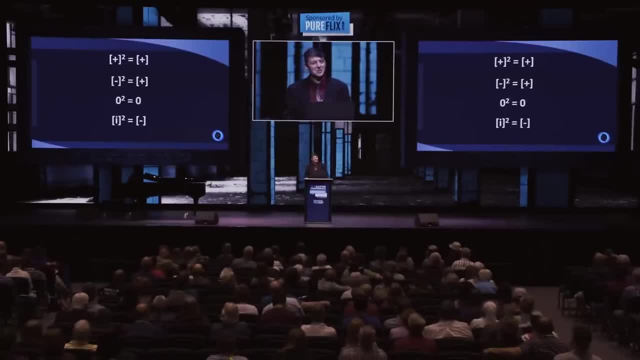 it's not zero, and that leaves us kind of scratching our heads a little bit. We have trouble with that. Well, I got news for you. Not everything in this universe is intuitive. If you've ever had a class in quantum mechanics, you know the universe doesn't work always the way. 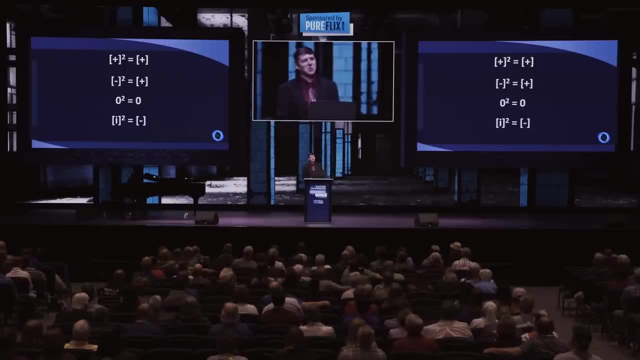 that we expect it to. You know, our intuition really is based on experience, and the fact is most adults don't have experience with imaginary numbers and so they seem strange. But it's just, it's just a matter of experience. When you were a little kid, negative numbers probably didn't make. 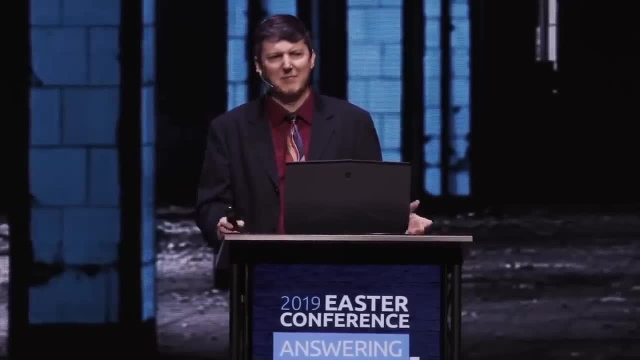 a lot of sense, right? You know I can have one apple, I can have two apples. How can I have negative two apples? That doesn't make sense. How can you have less than nothing? You get a little bit older, you get a bank account. 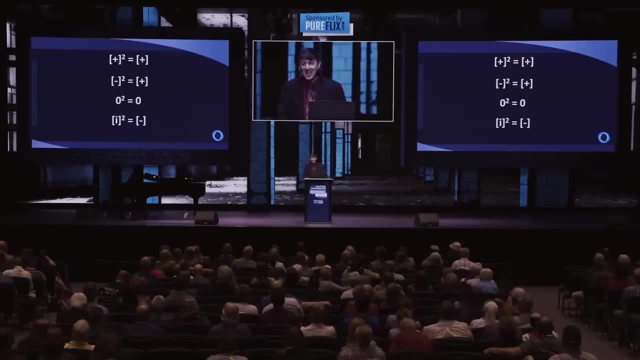 Suddenly negative numbers make a lot of sense, right? Yes, I can have less than nothing. Well, imaginary numbers are the same way. You gain a little experience and you find, yes, there are numbers that when you square them you get a negative, But they're not positive. 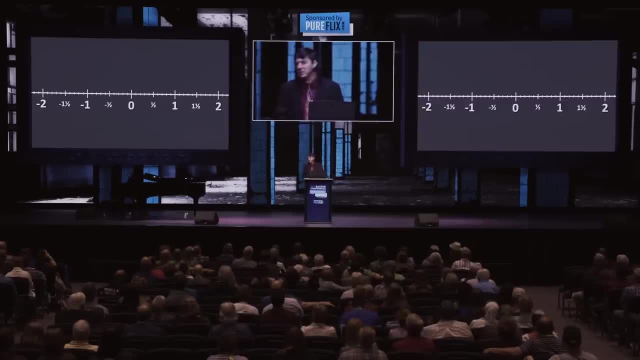 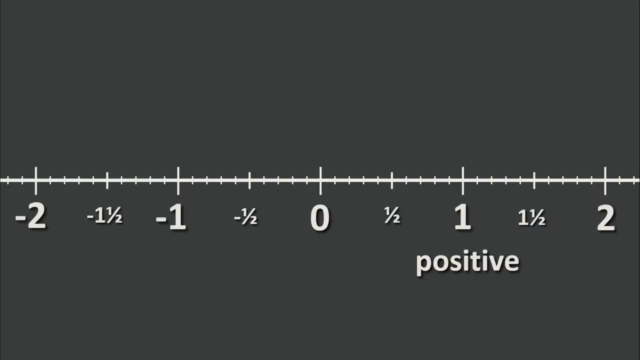 they're not negative and they're not zero. How do we make sense of that? One way to do it is if you consider a number line. So here we have a number line. Now the positive numbers are to the right of zero along that number line. The negative numbers are to the left. 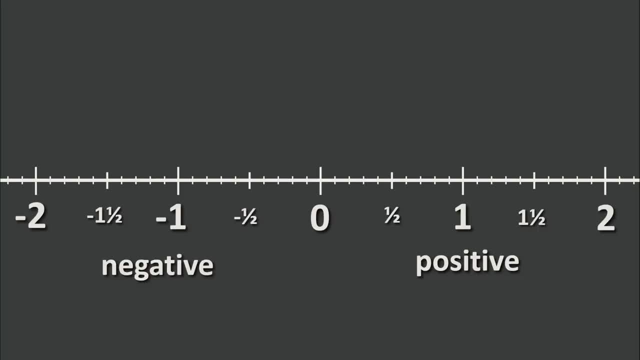 of zero along that number line. So how do we represent a number that's not positive, not negative and not zero? Well, you put it up above the number line, like that. It's not on the number line, It's on a different axis, And by multiplying i by the other real numbers, you can. 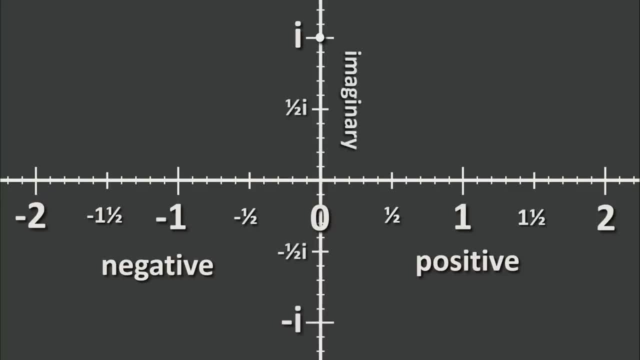 have all kinds of imaginary numbers. You can think of them as being on a different axis. So the real numbers are along this axis, The imaginary numbers are along that axis. Doesn't that make sense? You can see that the imaginary number it's not positive because it's not to the right of zero. 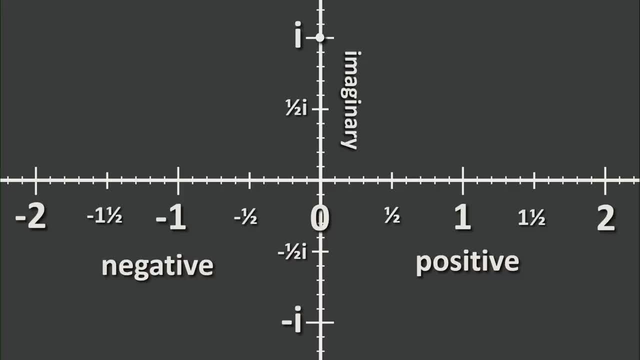 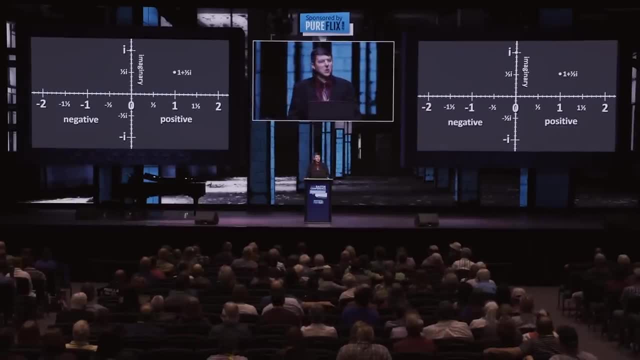 It's not negative because it's not to the left of zero and yet it's not zero. That kind of makes sense. And then you can also have numbers that are called complex and they're off axis. They're called complex because they have a real part and an imaginary part, But it's one. 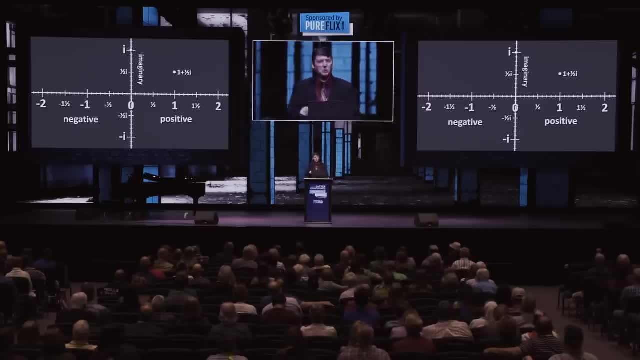 number with two parts, and usually the real part is represented by the x-axis and then the imaginary part is represented by the y-axis, And so you can plot any number in a plane by those two components, the real component being the x and the imaginary component being the y. That's kind. 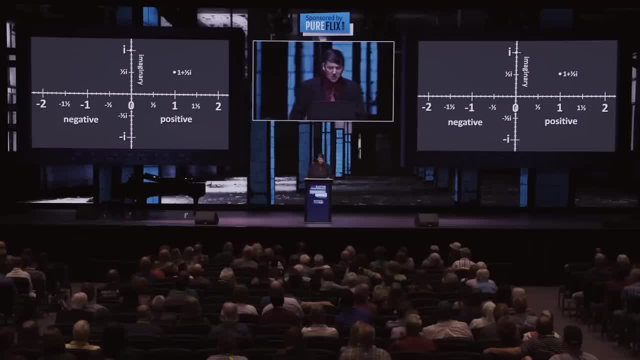 of neat. I can represent that. I can represent any number on a plane, Very convenient. So the Mandelbrot set also includes these imaginary and complex numbers. And the only thing you need to remember, they obey all the ordinary rules. 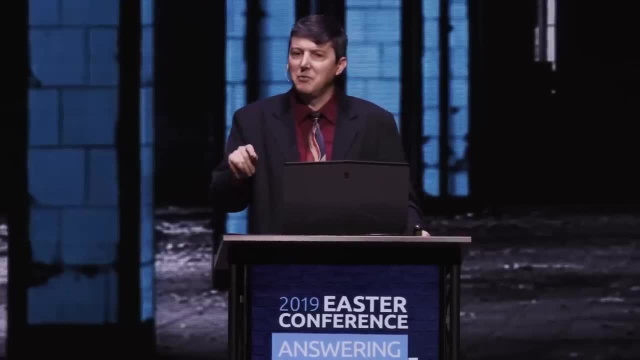 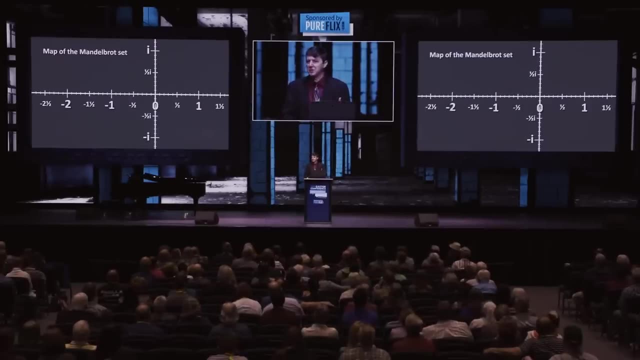 of algebra. It's just that when you multiply i by itself, you get negative one. That's the only thing you have to remember. What we can do then is we can make a map, because I'm trying to figure out if there's a pattern to the numbers that belong to the Mandelbrot set. And it turns out there is, But it's. 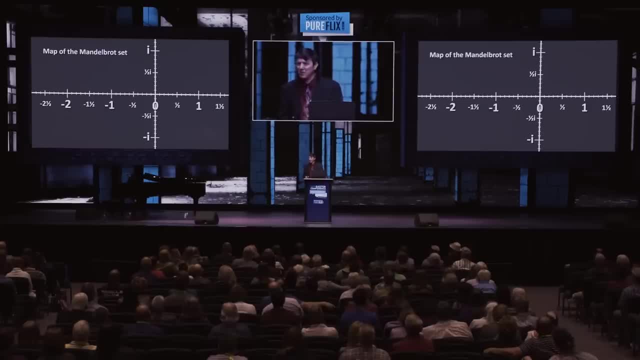 not obvious, right? Because you can't tell just by looking at a number whether it's going to belong or not. You have to run it through that formula and that's kind of tedious. But in the 1980s computers were starting to get fast enough where they could. 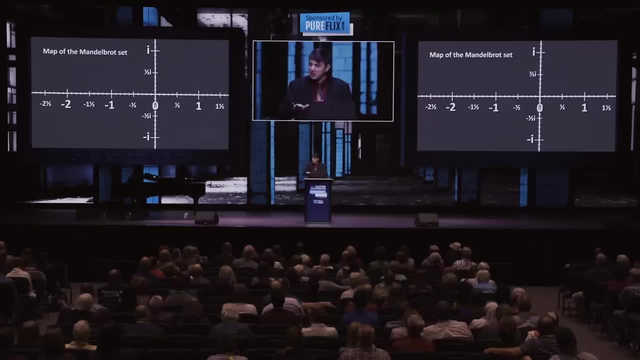 iterate that formula a number of times and they could analyze to see whether z is getting big or staying small. And so what we can do is we can have the computer check all these different points and we'll see if there's a pattern to the 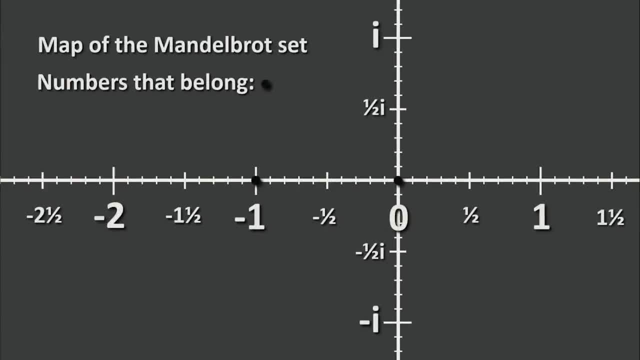 Mandelbrot set, And so we'll take the points that belong to the Mandelbrot set and we'll color those black. That's arbitrary. That's the way Benoit meant it. Benoit Mandelbrot did it, and we follow his example And you have the computer check more points and you find that all those 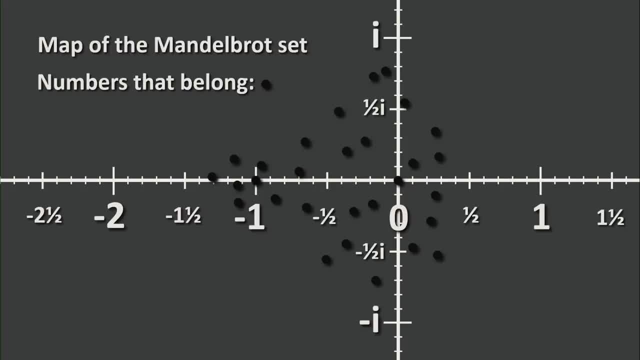 points right there belong to the Mandelbrot set. When you run it through, that formula z stays small. And then the points that do not belong. we'll color those red or some other color, It doesn't really matter. And so we already checked the point one. We found that 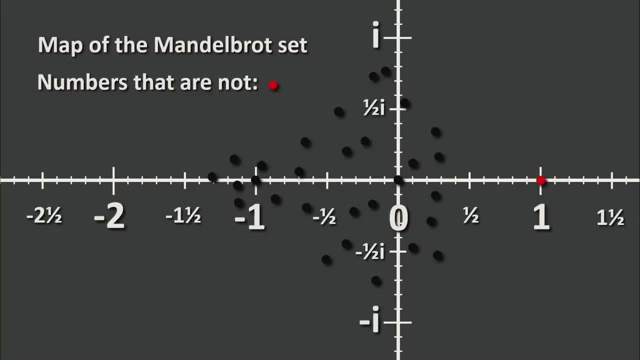 the number one does not belong to the Mandelbrot set, so it gets colored red. And had we checked these other points, we would find that they do not belong. And so you see, as you plot more and more of these points, pattern starts to emerge. 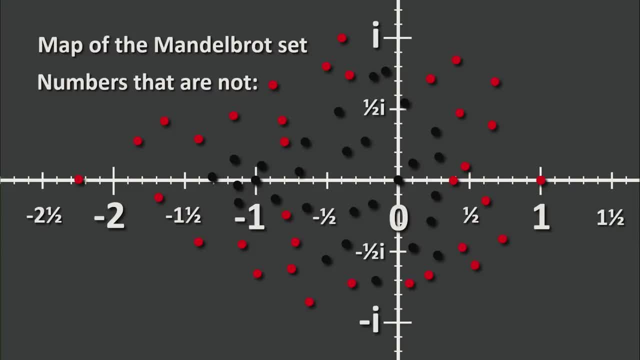 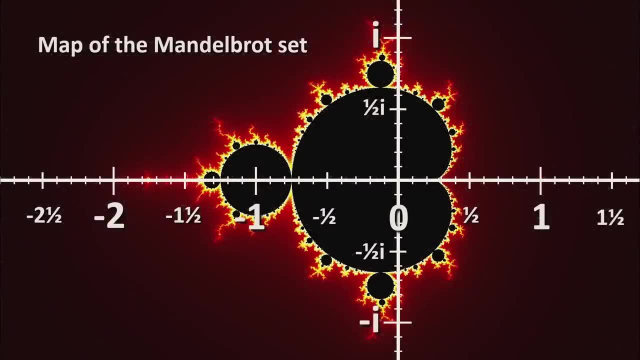 What's it going to look like? Well, you have the computer run through thousands and thousands of points. You have the computer check each one of those numbers and a pattern emerges. And the pattern looks like this. It's really interesting and unexpected. 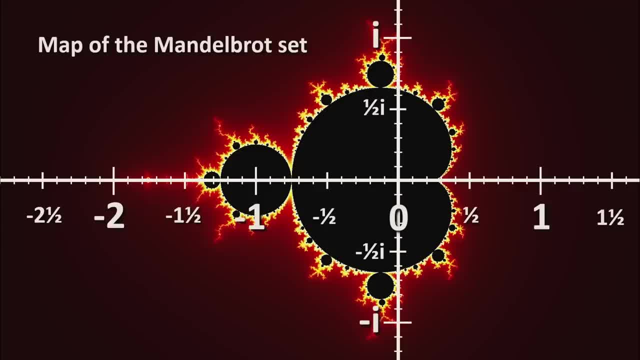 Nobody was expecting that when you made a map of the Mandelbrot set it would look like that Remarkable. I'm going to remove the axes now because it turns out the shape is remarkable. I'm using it for a very nice. and I tell you it's additional noun, so you can't say that every other way. But anyway, it's a pretty nice template And so I'm going to move around this and I'm letting our app host finish my task here. Now you can see I have a verbal guide thatbaum on this chart showing you. 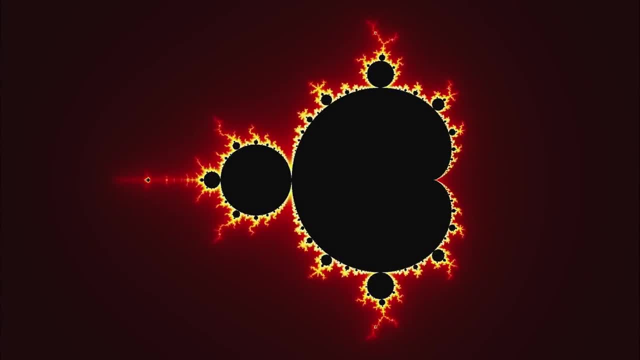 The shape is remarkably interesting and unexpected, and it'll turn out to have a lot of beauty in it as well. The shape itself is. I mean, this is a mathematical plot. I guess we'd expect it would have some mathematical properties to it, but everyone was surprised by the properties it has. 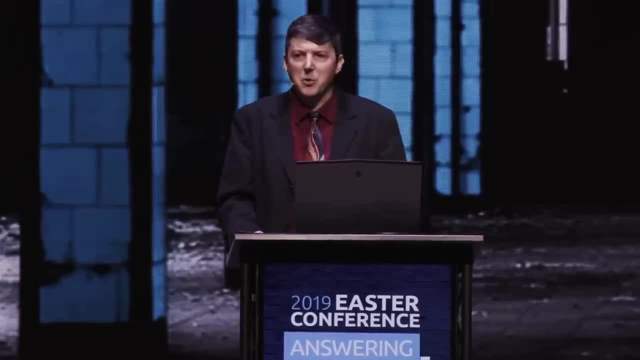 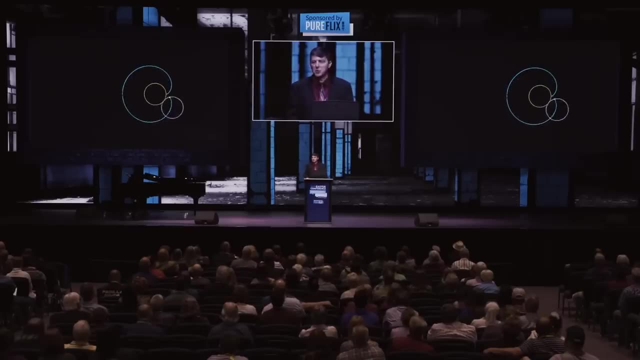 The main shape that looks kind of like a heart, that's called a cardioid. and a cardioid is what happens when you take a circle and you take your pencil on it and roll it around another circle of equal size. The shape you'll get is a cardioid, and you can see that, sure enough, the main part of 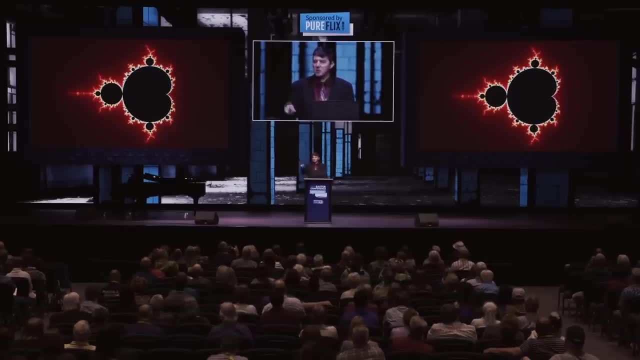 the Mandelbrot set is a perfect cardioid. All the other shapes that are growing off of it are circles, all these perfect circles attached to the perimeter of the Mandelbrot set. and then you see some other features, like these little tendrils that grow off of it and a spike over on the left, kind of that. 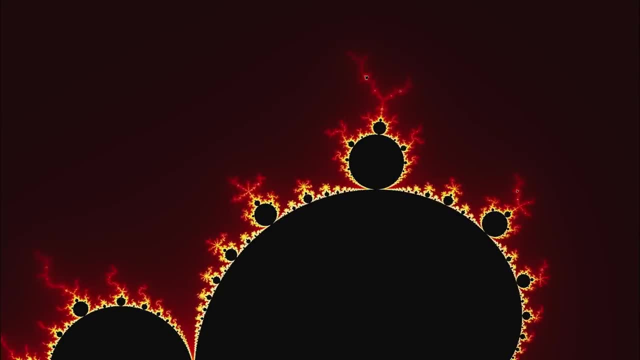 juts out. That's kind of interesting. You notice that top circle there. it's got a circle on top of it, another one on top of it on smaller and smaller scales and it goes out and forms this little tree and it's. 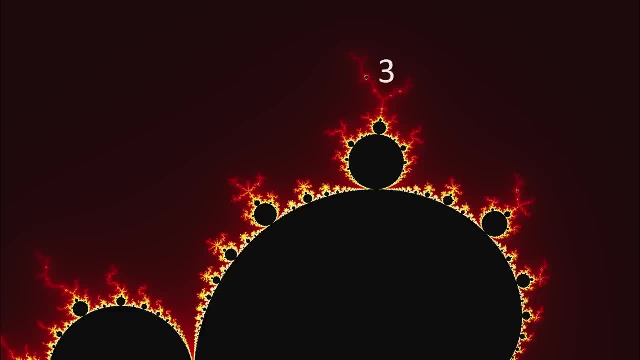 got three… three stems to it, including the trunk. so it's got a trunk and two stems for a total of three branches. You see that there. Now the next one to the left branches into five, Can you see that? I mean it's kind of small, but you can see the five branches there. 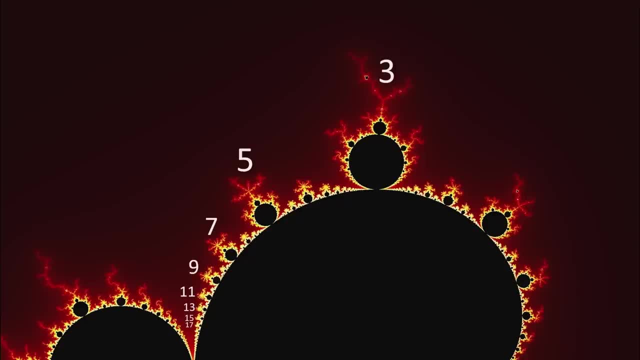 The next one is seven, nine, eleven, thirteen, fifteen. It's all the odd numbers, And, by the way, they don't stop. they go to infinity. There's an infinite number of them. They get smaller and smaller, though, and so you have to zoom in more. 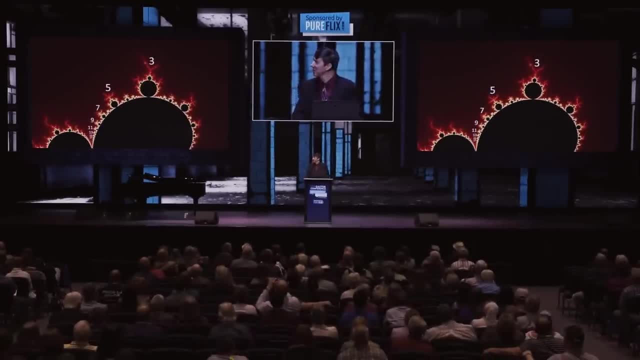 But all… all the Mandelbrot set knows how to count. It's kind of remarkable. And then on the other side, you have the odds and the evens. You have all the numbers there in terms of the number of branches. 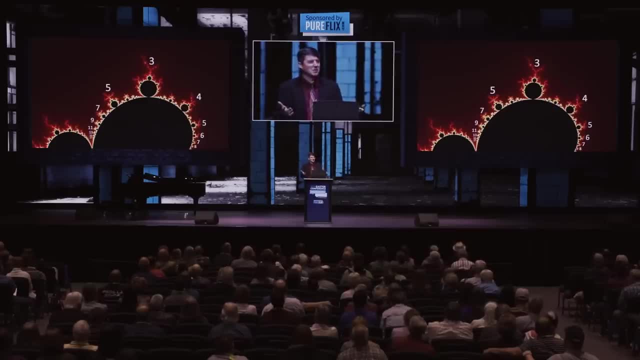 Now it's remarkable enough that they have branches at all, because who would have thought that when you run numbers through that little formula, you get that shape. It's remarkable, Nobody was expecting that. And it's even more remarkable that it has the ability, apparently, to count in terms. 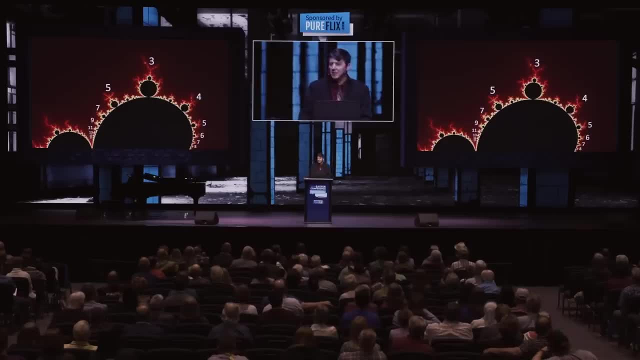 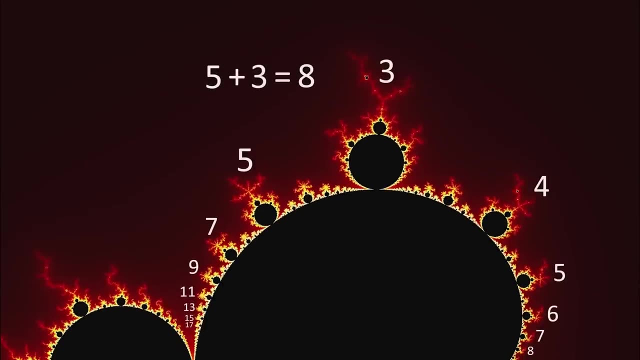 of the number of tendrils that grow off of each… each bud there. And of course you can take two of those, Those numbers like five and three. you know five plus three is eight, okay, And it turns out that the bud in between those two has eight tendrils. 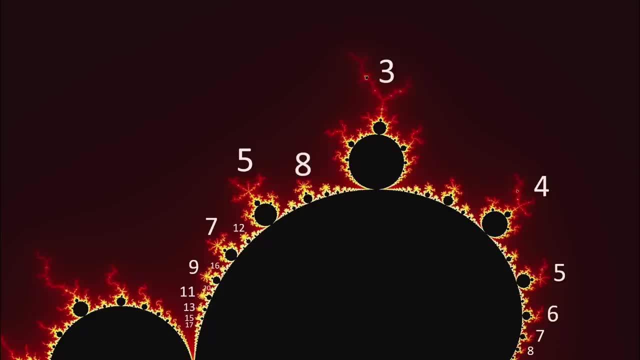 Interesting, And that's true of all of them, both on the left side and the right. The bud in between the two adds the number of tendrils on each one. So not only does the Mandelbrot set know how to count, it knows how to add. 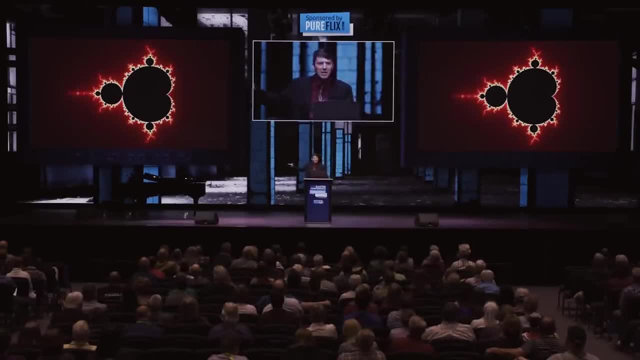 And then on the… on the left side over there, you've got this kind of spike that goes out And you see there's this little bump on the end of the spike. So let's take a look and see what that looks like. 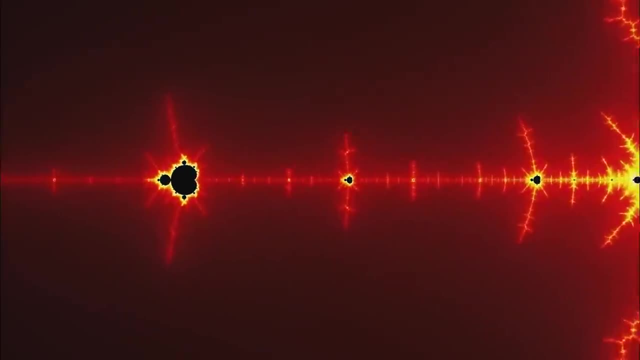 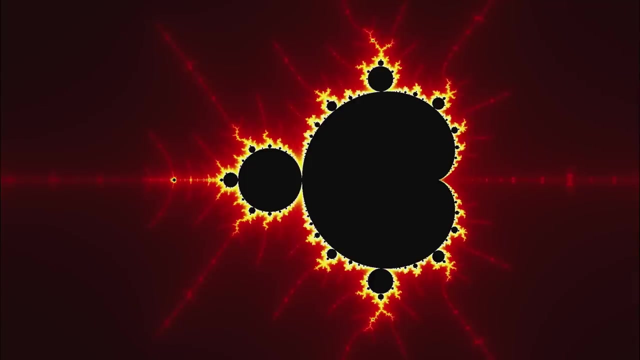 So we'll zoom in on it And that little bump turns out. it looks like the entire Mandelbrot set. It's a… it's a mini Mandelbrot set And it's almost identical to the parent, except it's got extra spikes growing off. 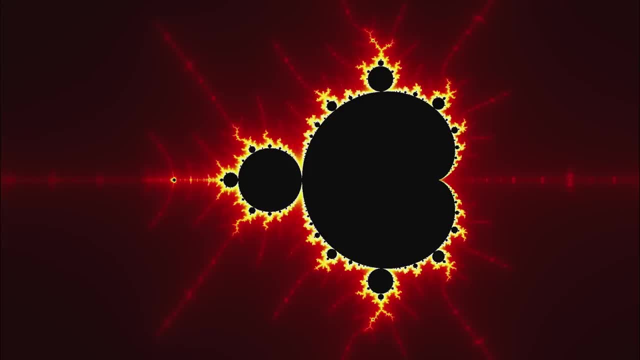 of it, But the basic shape's the same. It's got the cardioid and the circles And, oh, it has a little spike growing off of it too, with a little bump. What could that be? Well, let's zoom in on that. 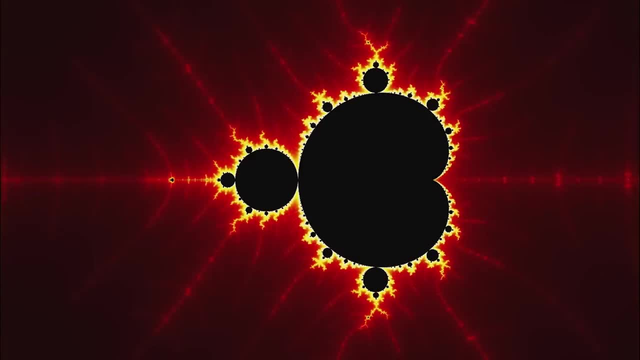 And oh, interesting, Absolutely fascinating. It's got extra spikes growing off of it And that's got a little bud. How about that? Now, of course, you could do that literally forever, And it…. there's an infinite number of baby versions built into the Mandelbrot, set on smaller and 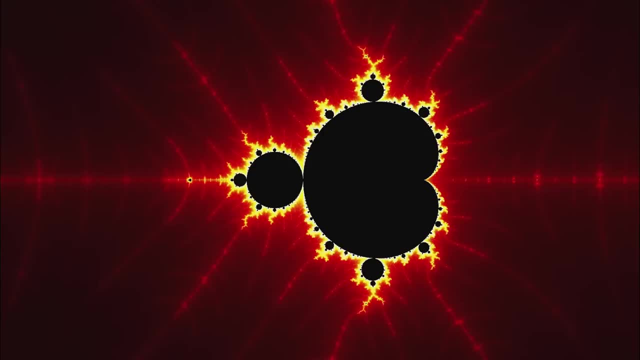 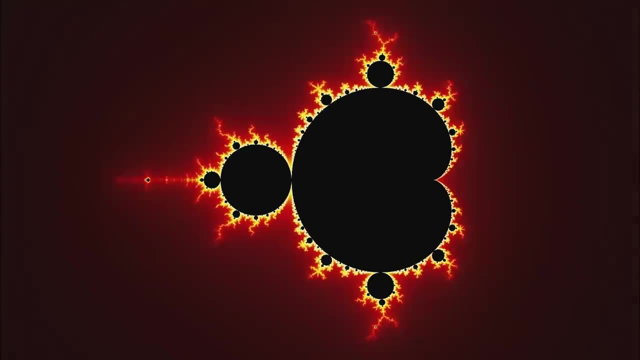 smaller scales And take a look at how small this is compared to the original. when we zoom back out here, Look at how tiny it is. Isn't that remarkable? And the fact that it repeats infinitely and it doesn't lose complexity- it actually. 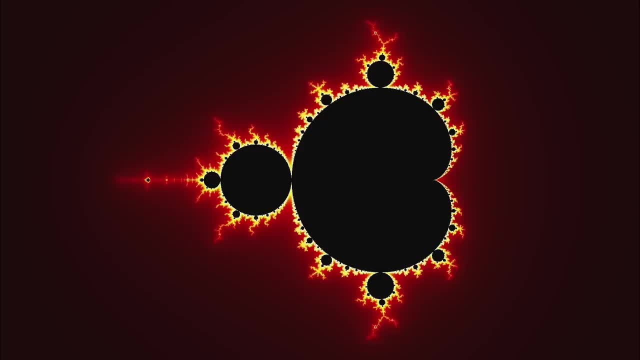 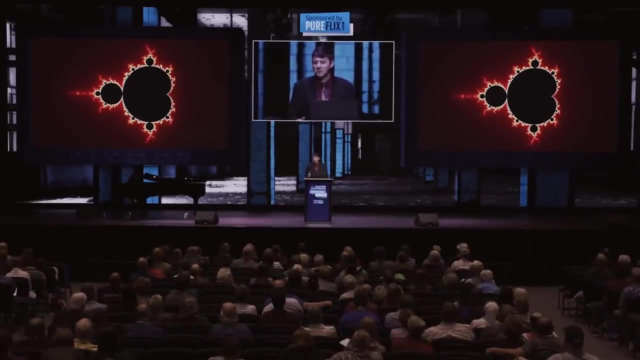 gains it each time you get extra spikes growing off of it. Very remarkable. Well, to anticipate my conclusion in this, I'm going to suggest to you that this shape tells us something about the way God thinks. God's understanding is infinite. Numbers are an aspect of God's mind. 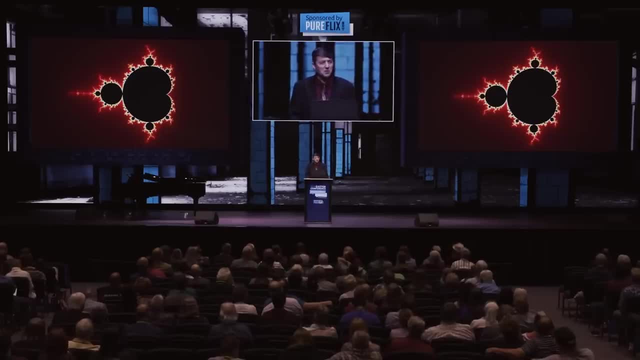 God is responsible for numbers, And so it makes sense in the Christian worldview that when we… when we explore and study numbers, we should… we find intelligence in them. We find evidence of patterns, And not only just… not only intelligence. We find infinite intelligence, because this thing repeats infinitely. 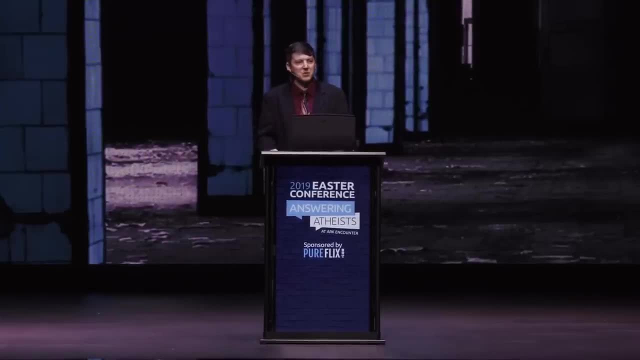 A structure that repeats itself on smaller and smaller scales is called a fractal. So the Mandelbrot set is one example of a fractal. There are other types of fractals. There are other sections of the Mandelbrot set that are fractal. 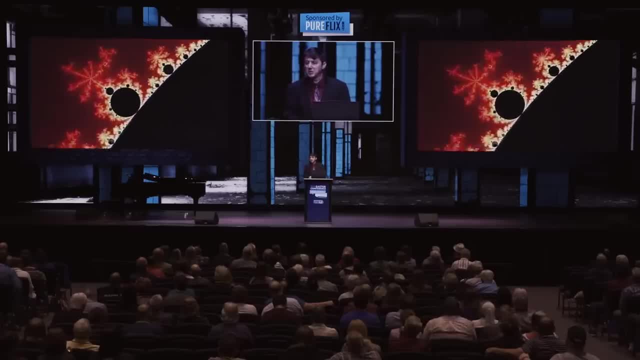 We could zoom in, for example, on one of these little tendril features here and zoom in on that and you'd say, well, that's interesting, We'll just… you think what's going to stop at some point, right? 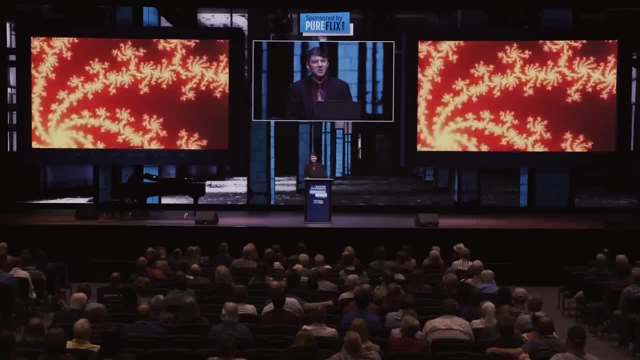 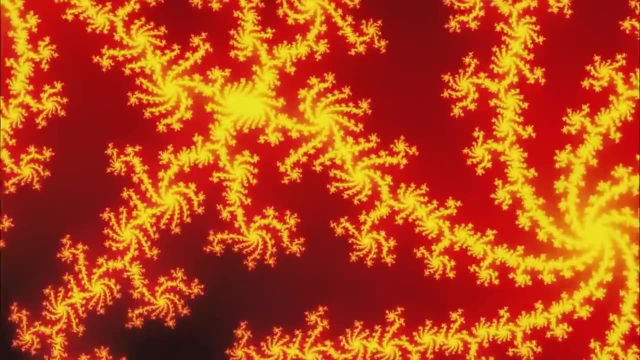 Eventually it'll even out and you'll get… but it just keeps going. It's infinitely wiggly. you see That little… it's wiggling around like that and you zoom in on it and it keeps going and keeps going and keeps going. 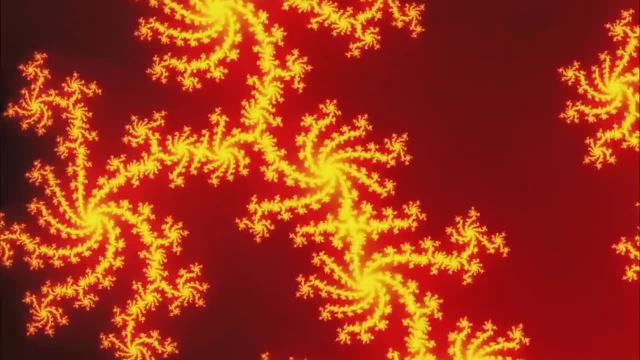 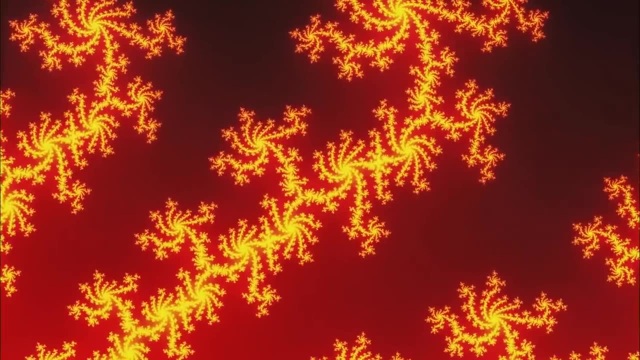 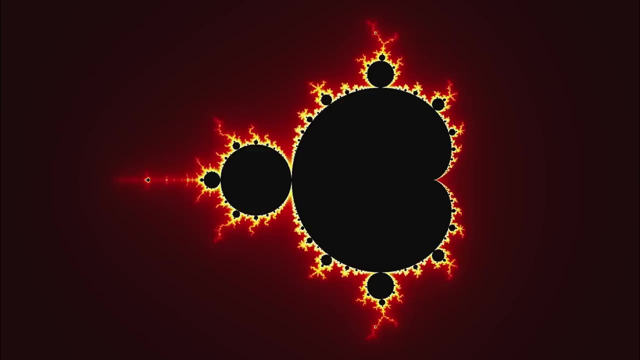 It's just mesmerizing to watch this thing and see the scale here, and it gives you a little taste of what God's mind is like to be able to think infinitely. We can only process just a little bit of information at a time, but God's mind is truly infinite. 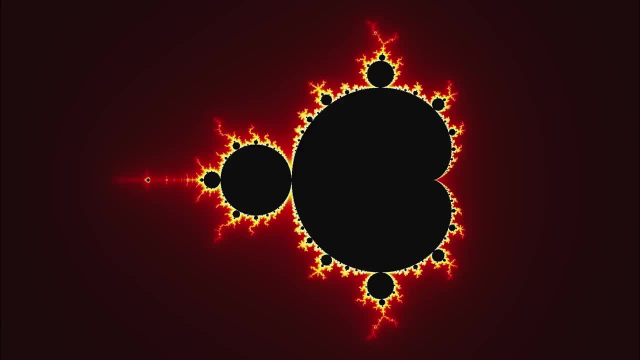 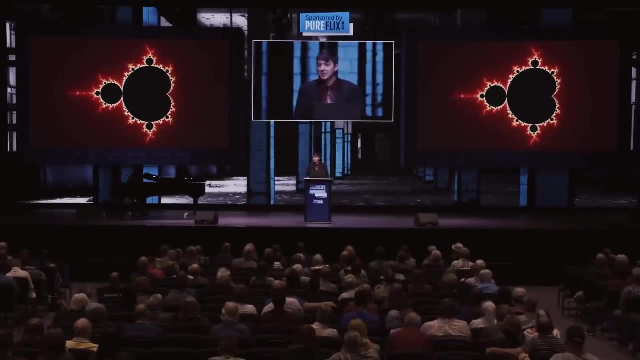 So one of the interesting areas to explore… and what I want to do now is just kind of spend some time exploring this shape that exists in the mind of God and has existed in the mind of God from creation that was only discovered in the 1980s. 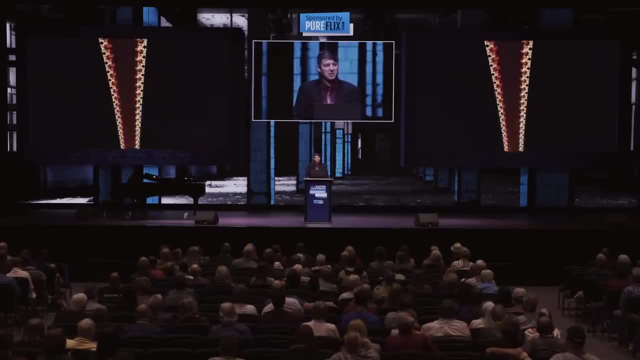 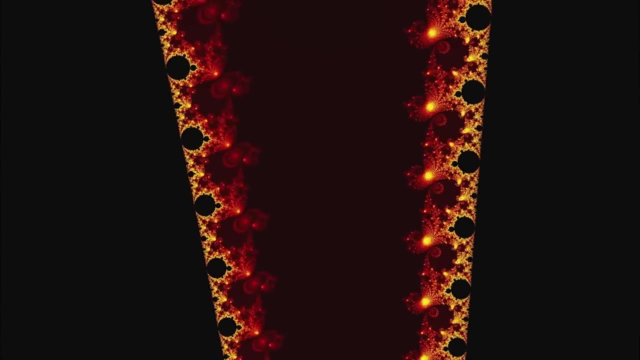 And we can zoom in, for example, on this cusp between the main cardioid and the disc and we find it's called… they call it the Valley of the Seahorses because you see over on the right side it looks like seahorses. 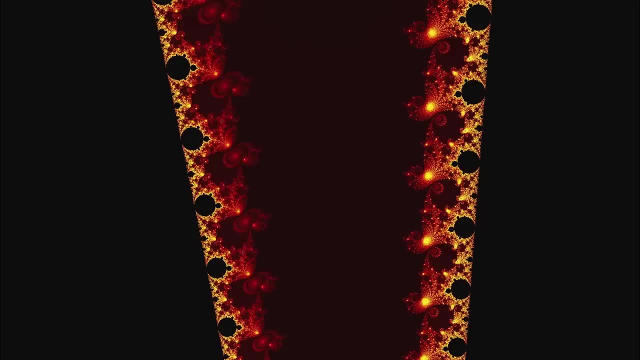 They're upside down because of the way we've zoomed in on them here. Now the colors are arbitrary. I can make them whatever I want and we'll change them every now and then just to keep things interesting. But just keep in mind black always represents numbers that do belong to the Mandelbrot set. 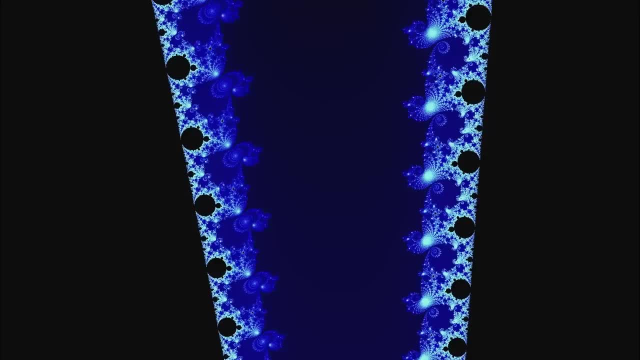 and then colors represent those that do not belong to the Mandelbrot set, And bright colors are very close to being on the Mandelbrot set, but not quite a part of it. So let's zoom in on one of these seahorse structures over here. 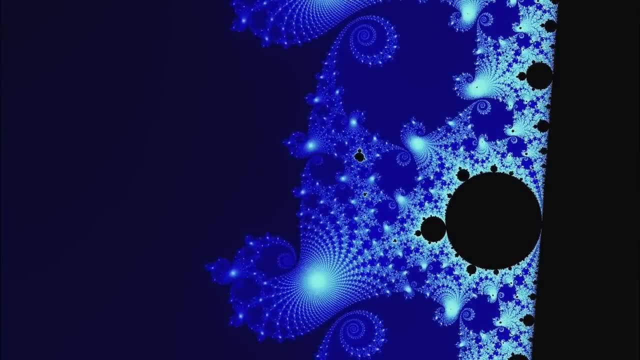 You see, it looks like an upside-down seahorse. Isn't that fascinating? Quite beautiful. And I need to explain a little bit about what this means, because if the points are very bright, that means it's very close to the Mandelbrot set and you might look and say: 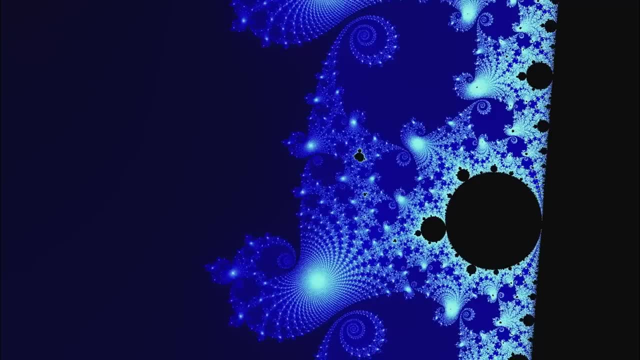 yeah, that bright hub doesn't look like it's anywhere close to it. It is. It's just. you need to realize that there is a very thin black thread that's wiggling around and making that shape. you see, It's just so thin. it's thinner than the pixels that the computer can plot. 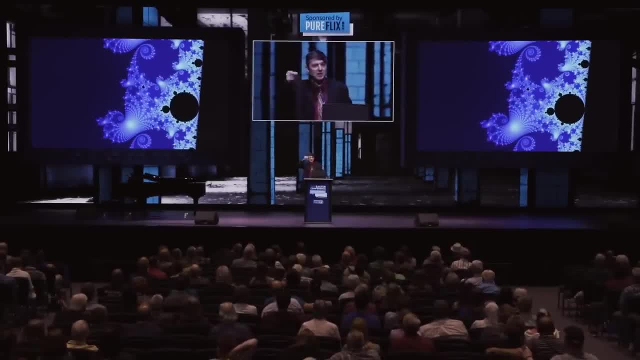 So everywhere you see structure like that, there is very thin black thread that's winding around and creating that wonderful shape. We'll zoom in and find out what this seahorse is made of. It's the central hub there. It looks kind of like a kind of like a spiderweb-type structure, right? 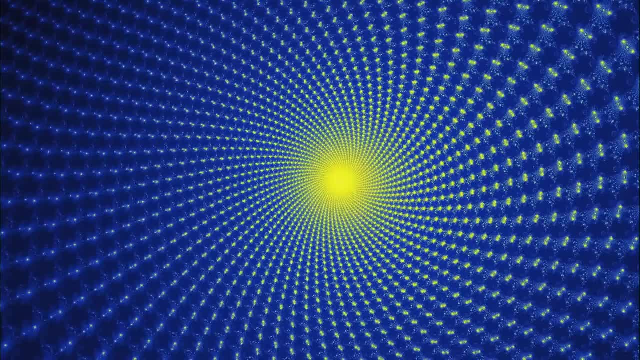 You got the spokes and the rims around there And I found from experience you can zoom in on the center of that until your heart's content and it doesn't really change very much. It goes on infinitely. So again, the infiniteness of the mind of God. 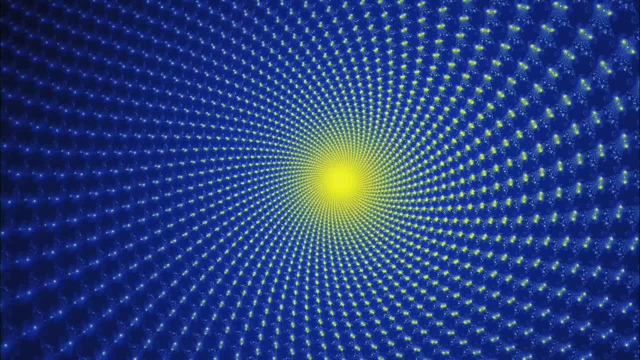 And so I thought, well, okay, let's go off to the side and figure out what the strands of the spiderweb are made of. So let's go off to the side here, and we find that the strands are made of more spiderwebs. 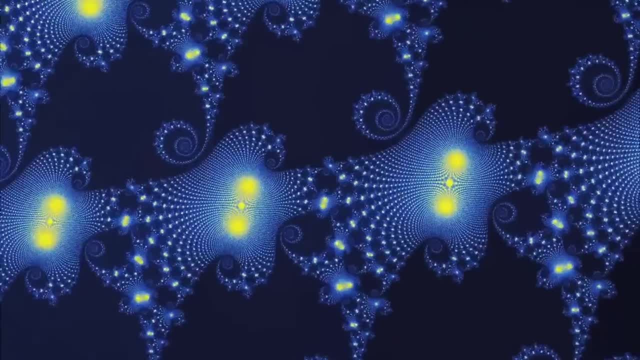 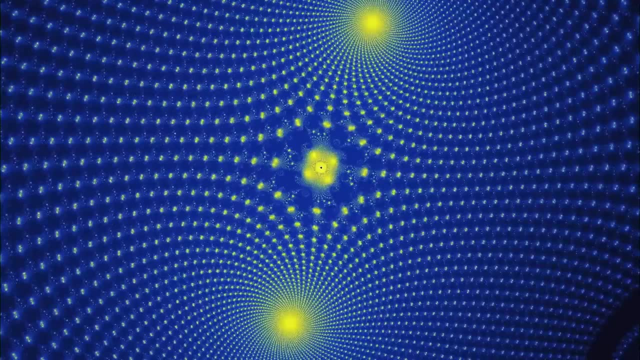 which is kind of interesting. And we zoom in a little bit more and you find that there's sort of two hubs there. You see the bright yellow hubs, And then in the middle it goes from two to four and as we zoom in it'll go from four. 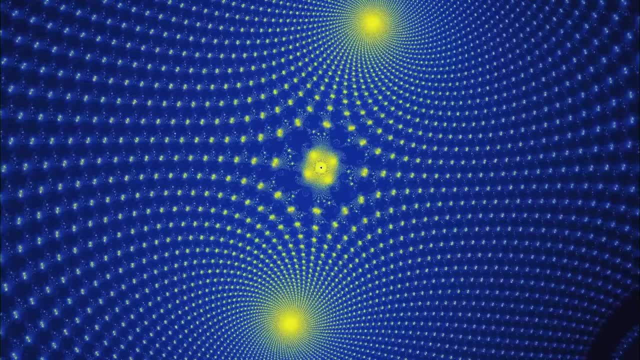 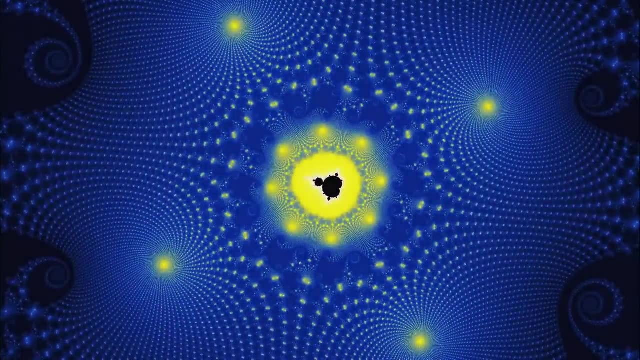 to eight, to 16,, 32,, 64, it doubles each time. And as we zoom in on that central hub, we find: oh, isn't that interesting. You see it going from four to eight, to 16, and so on, and in the middle, of course, you. 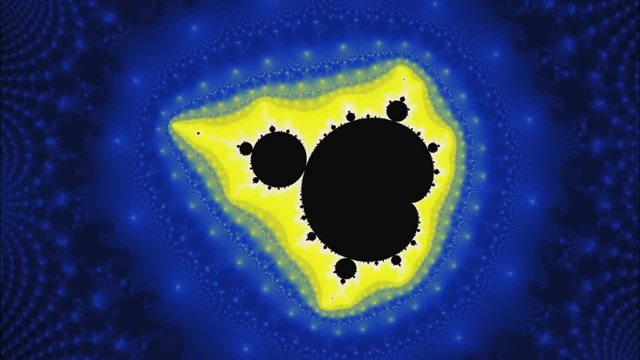 have another baby Mandelbrot set. Quite fascinating. And again, there's an infinite number of these babies built into the overall shape, which I think is amazing. And again, look at how small this is compared to the overall shape as we zoom back out. 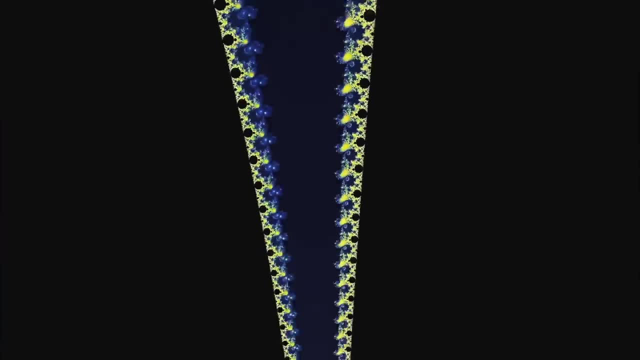 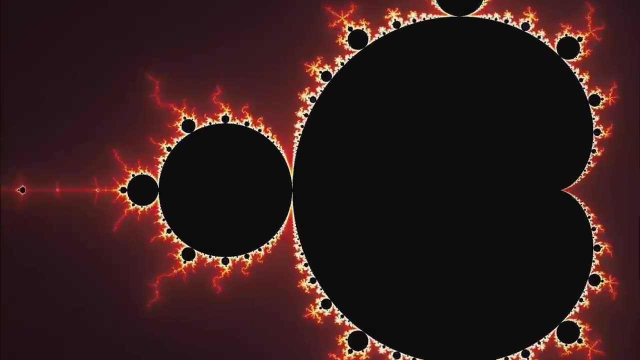 It's just a tiny little infinitesimal and we could have zoomed in on any one of those strands. I just picked one at random and there it is So pretty remarkable. Let's go back to that valley Now. the valley of seahorses is on the right. 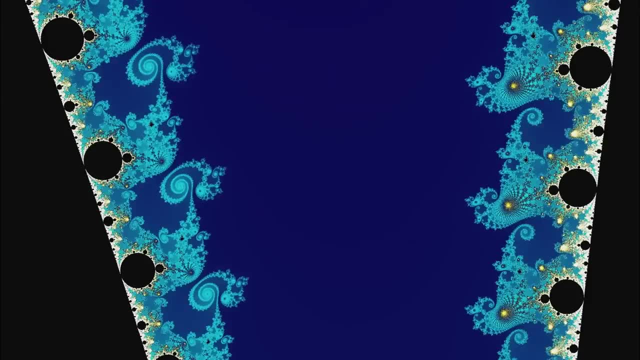 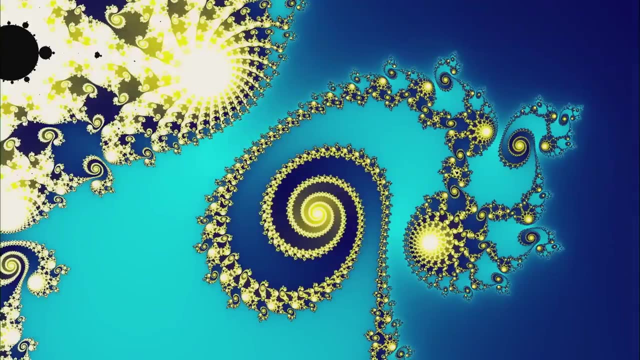 On the left we find the valley of the double spirals, And I'll zoom in on one of those now. This is my favorite part of the Mandelbrots, but I think they're very beautiful. They remind me of spiral galaxies actually, which, as an astronomer, I really appreciate. 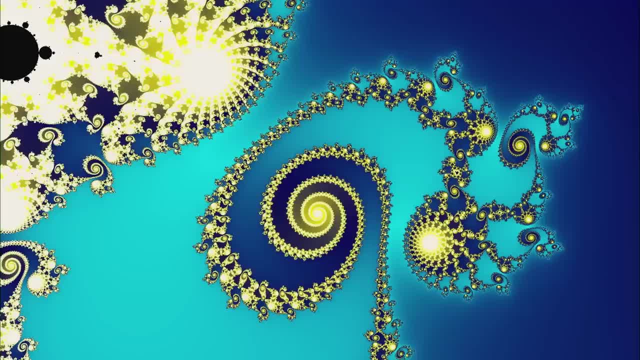 God apparently likes spirals because he's built a lot of them into nature and he's built them into math, which is remarkable. Who would have guessed that there would be a spiral, a beautiful spiral, built into that little formula, Z squared plus C, rather built into numbers when we run them through that? 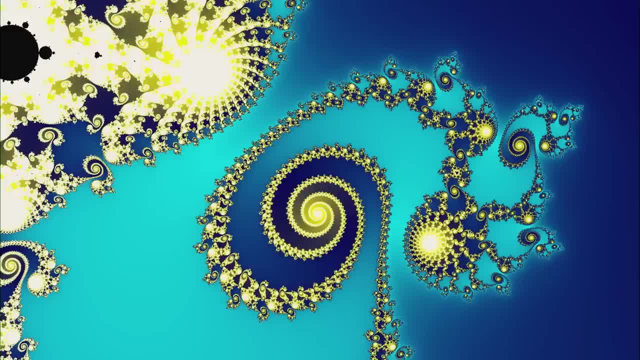 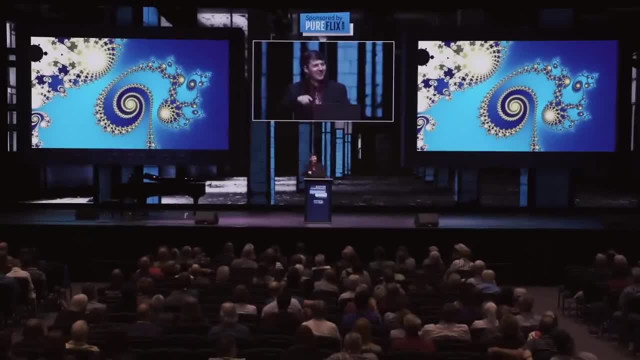 formula Pretty amazing. It's a double spiral because there's actually two strands that wrap around each other, wrap around each other. if you trace one strand, you'll find that it there's a strand in between, and so it is a double spiral, as our spiral galaxies, by the way, 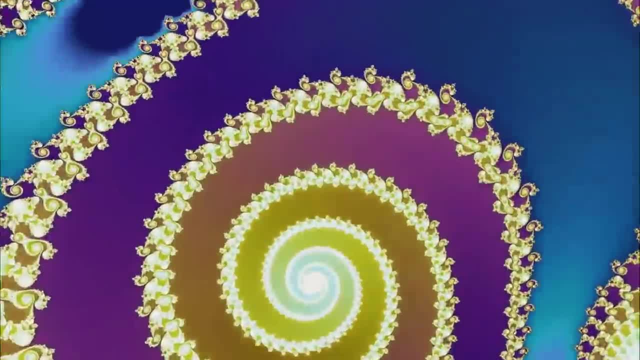 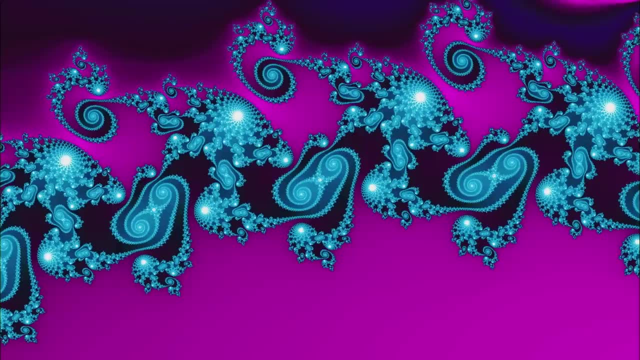 and let's zoom in on that a little bit. and again, I found you can zoom in on the center forever, so we'll zoom in on the side and you find that you find the spiderweb type structures, you find more double spirals and you find a new. 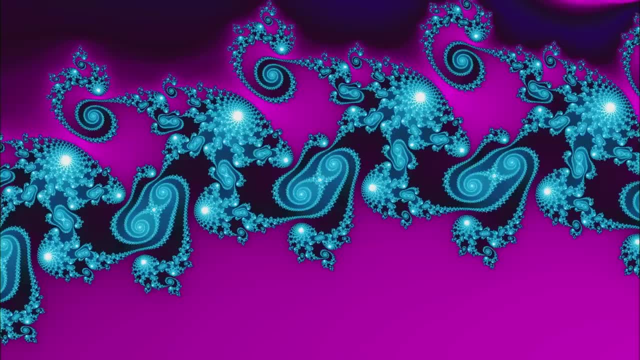 structure. I call them bow ties. they're kind of in the middle. you see, it looks like a, like a little bow tie right and it's got two double spirals that intersect in the middle. quite beautiful again what you're seeing here, the Mandelbrot set. it's just incredibly wiggly. it's so wiggly it's making these. 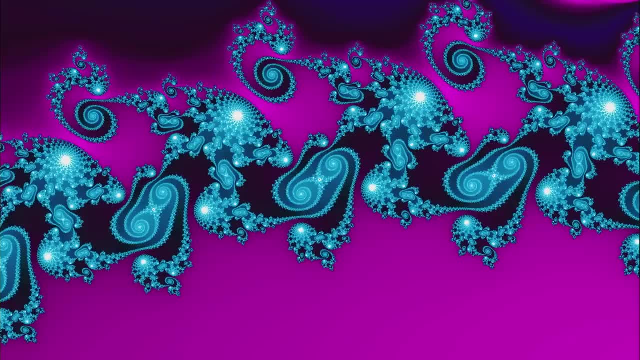 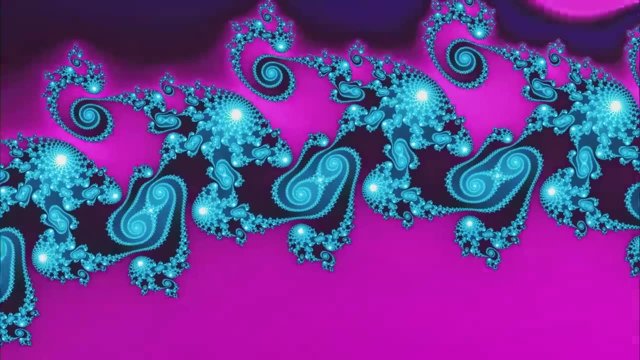 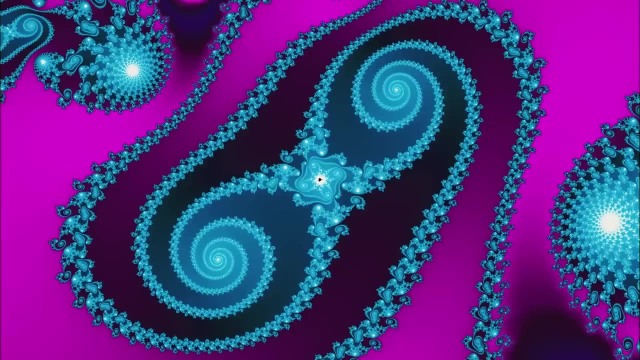 wonderful shapes and that's what the the points that are very bright are very close to that thin black thread that's wiggling around and making all these wonderful shapes. so we'll zoom in on one of these bow ties and we find that it's again. you have the two double spirals. we zoomed in on a double spiral and we 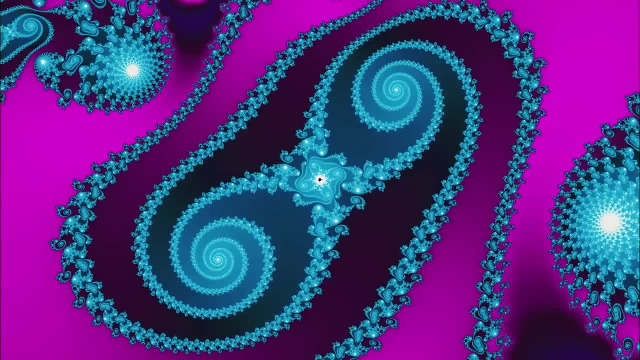 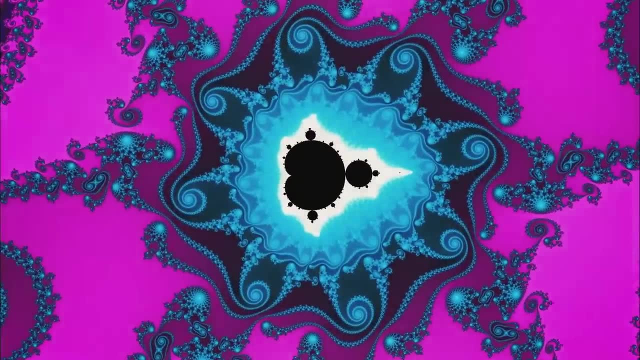 found that it's made up of multiple double spirals and they go from two to four to eight to sixteen. as we zoom in on the center, there and in the middle you find another mini Mandelbrot set. you're not surprised this time, but there it is, and 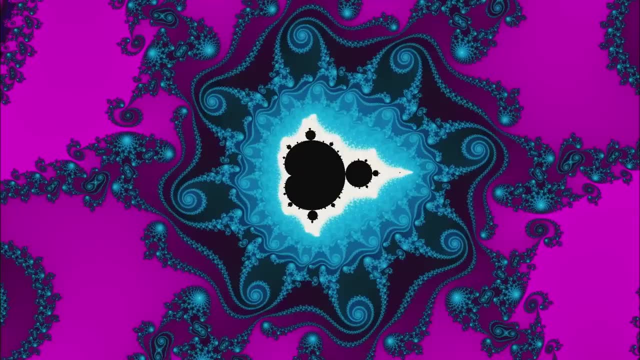 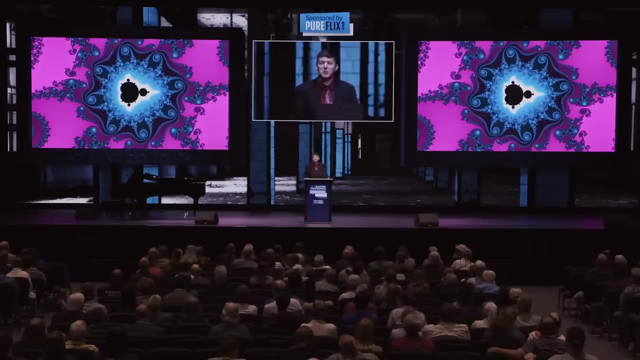 it quite beautiful. who would have imagined that such a beauty would be built into numbers? well, in the Christian worldview that makes sense. we serve a God who is beautiful, who makes beautiful things, and when we examine the way God thinks about numbers, which is what mathematics really is- 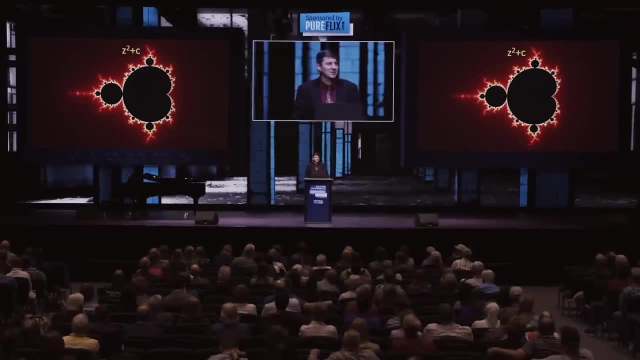 we find it's immensely beautiful. all that, just a map, a map of what numbers belong to that little formula when you run them through that algorithm. isn't that fascinating? and this, of course, was astonishing to mathematical mathematicians when this was discovered back in the back in the 80s. so then it. 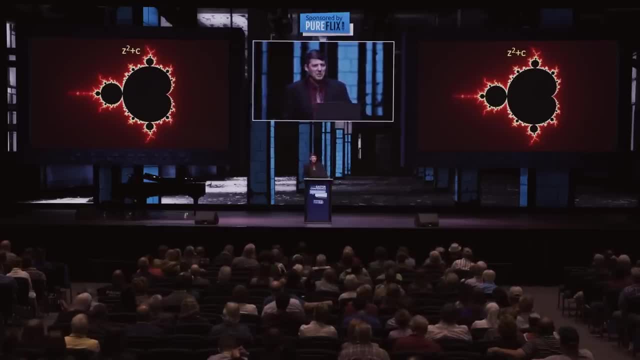 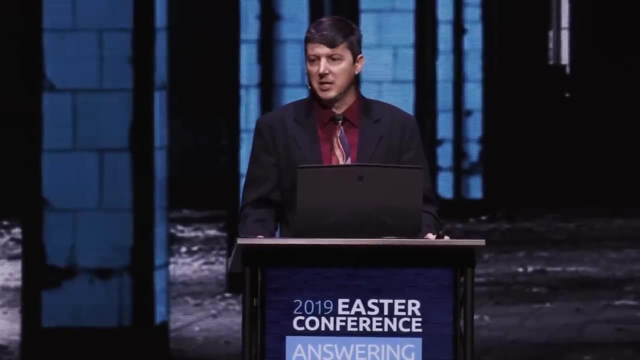 occurred to me: well, is there something special about that formula? I mean, did we just happen to stumble upon to the, you know, to an amazing formula? what happens if we change it? so I thought, okay, let's take what happens if we go Z tilde with a letter. 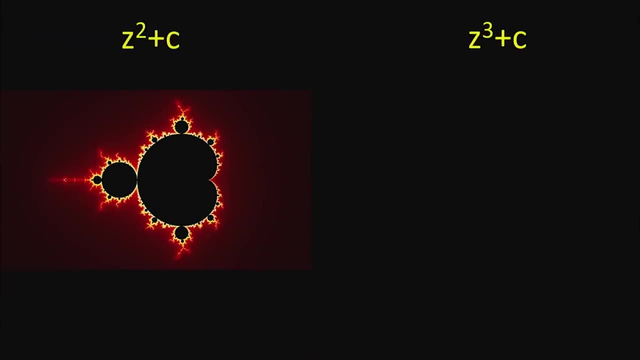 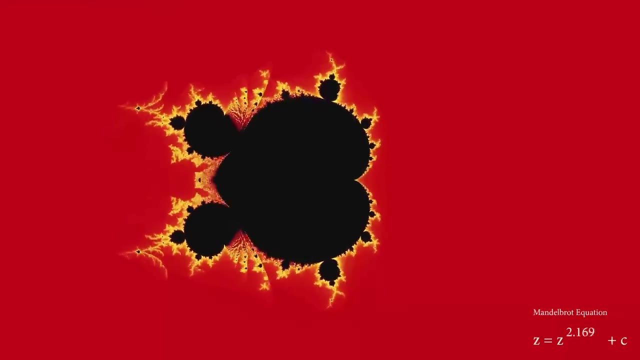 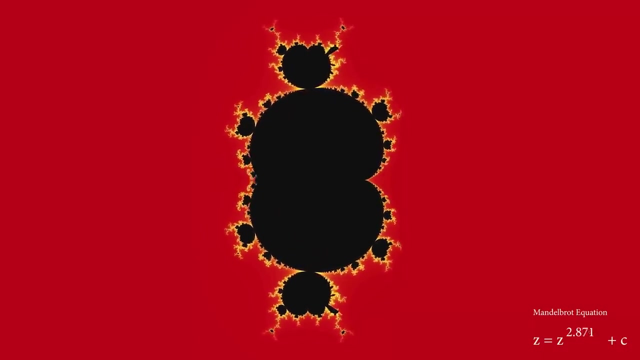 cubed plus C. Well, I ran the computer code through that and it turns out you get a different shape, Interesting And very similar in some respects but different in others. The shape here, the main shape, is called a nephroid, and nephroid is what happens when you take. 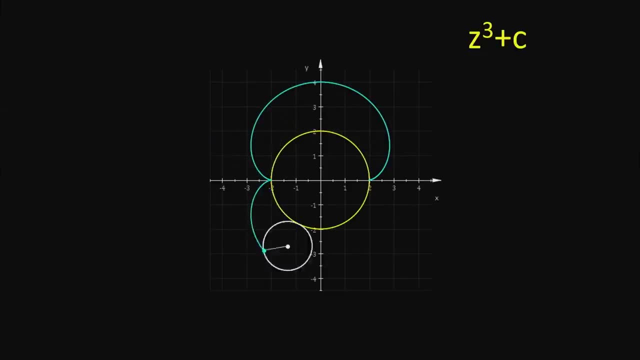 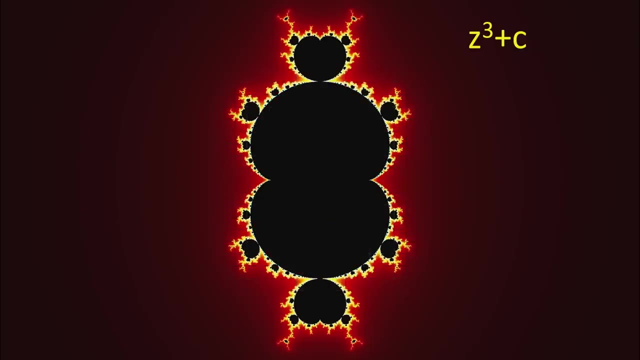 a circle half the size of another and you roll it around, then you get that shape And you can see it's a perfect nephroid, Really amazing. And then, instead of circles growing off of it, you have cardioids growing off of it. Notice, everything's gone up by one. 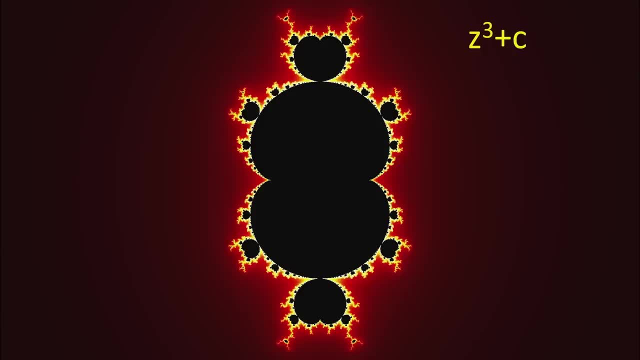 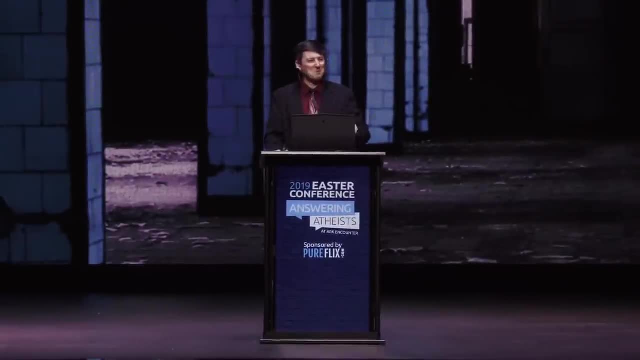 The Mandelbrot set had a cardioid which has one valley. This one has a nephroid which has two, And the circles growing on it which have no valleys now are cardioids which have one valley. Everything's gone up by one. That kind of makes sense. We went from Z squared 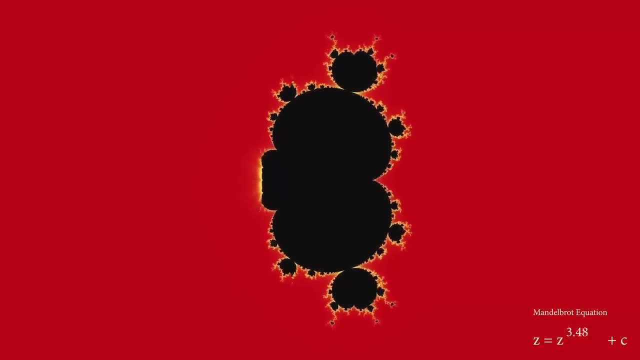 to Z: cubed. I guess that makes sense. Okay, what happens when we go Z to the fourth? Well, that's what you get. Okay, what happens if you go Z to the fifth Interesting? You notice the number of lobes. 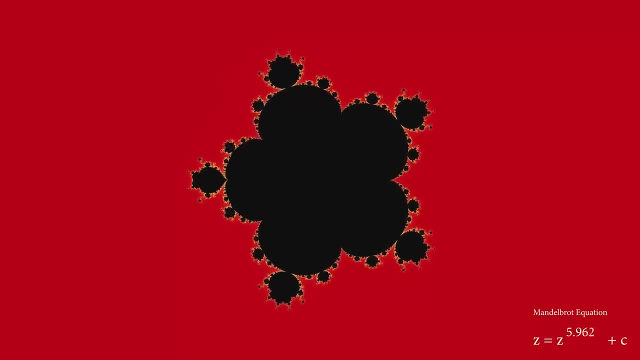 Okay, Okay. And what happens to the number of lobes? Is one less than the number? So, Z to the fifth, you get four lobes. Z to the sixth, you get five lobes. It occurred to me if I went Z. 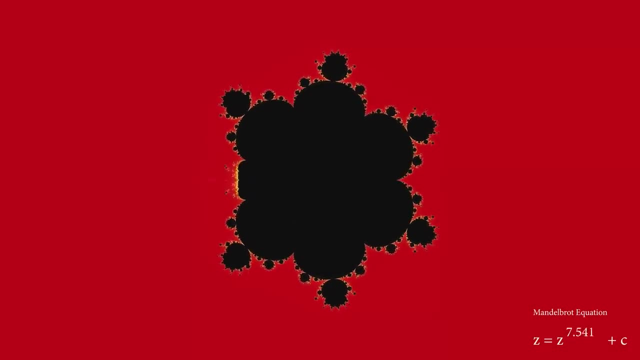 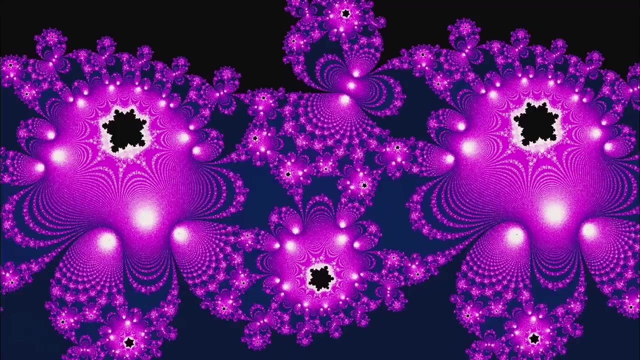 to the seventh, I could get snowflakes, And you sure do. And if you zoom in on it, do you get snowflakes? Absolutely You zoom in on it. you get snowflakes everywhere, Isn't that wonderful. Did you know that such a beauty was built into numbers? 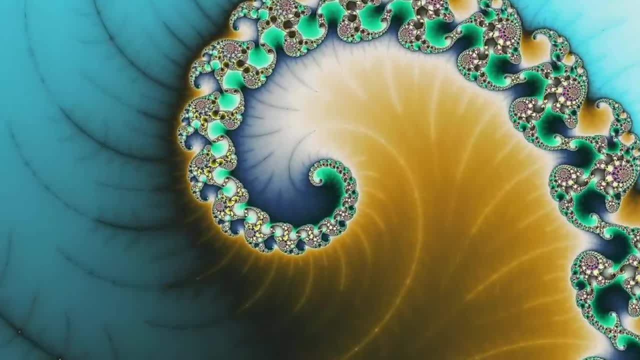 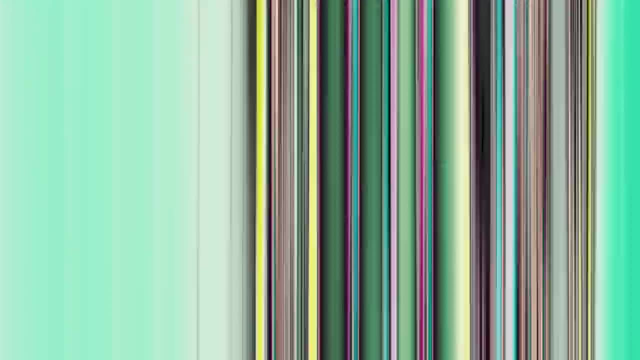 Okay, so what does all this mean? We've got these wonderful shapes and it's very pretty, Dr Lyle, but who cares? Well, I want to ask what causes the beauty in fractals, Because, I think you'd agree, they're beautiful, They're beautiful and they're. 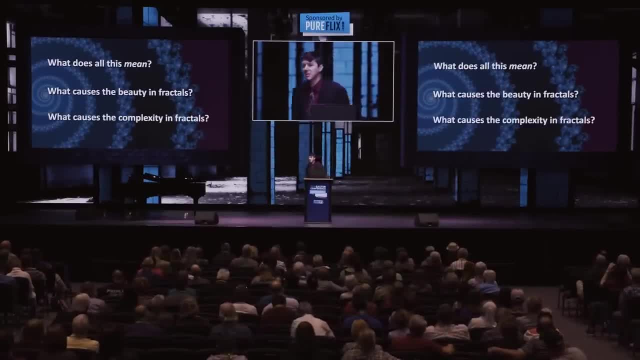 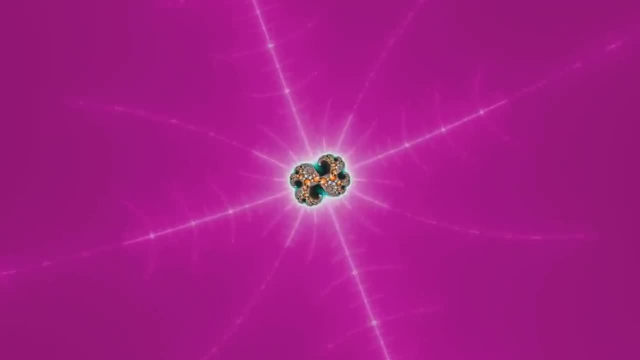 certainly complex, and so I have to ask: what causes the complexity in them? The fact that when you zoom in, you get not only baby versions, but the complexity increases as you zoom in rather than decreases. What's causing that? So let's answer the first one first. What causes? 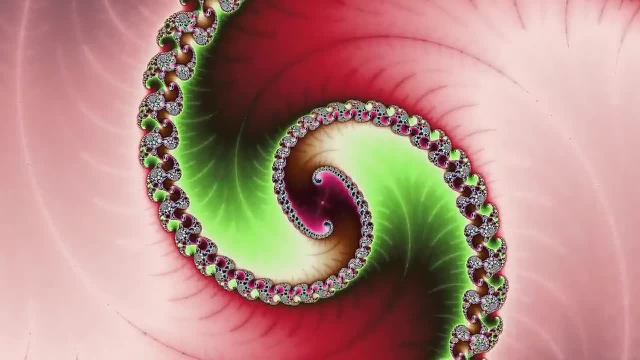 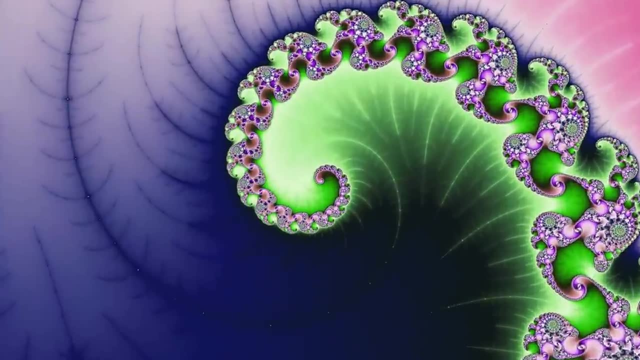 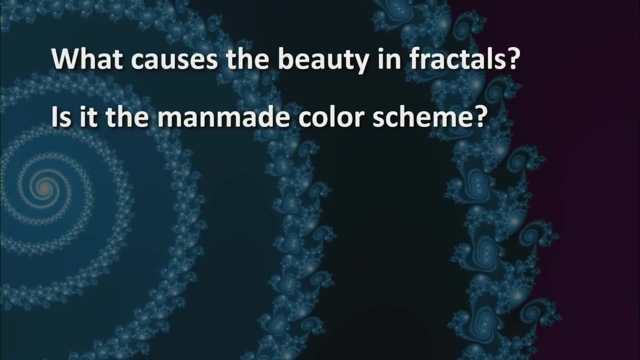 the beauty in fractals, And I'll have several possibilities. Could it be the man-made color scheme? Now, I told you that the colors are arbitrary. We always assign black to the set itself and then we assign other colors to the perimeter to make it easier to see. and I'll admit 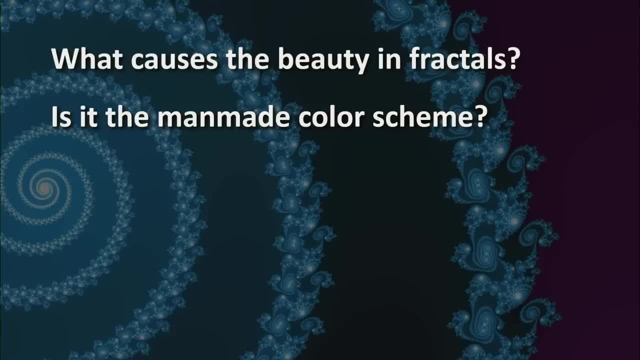 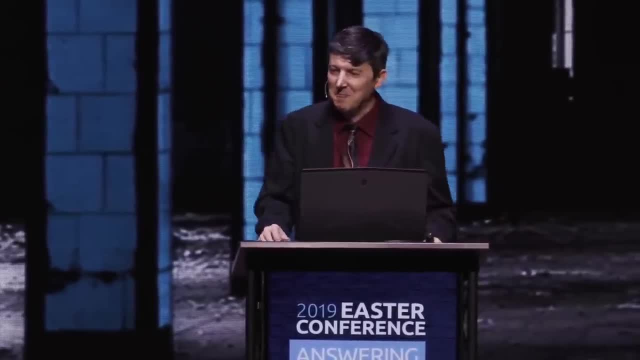 I picked the colors. I think they're pretty. Other people pick other colors, sometimes not always pleasant ones, and shame on them. because you know I do have an artistic side. I appreciate beauty anyway. Is it the man-made color scheme? I would say no because, although I think the 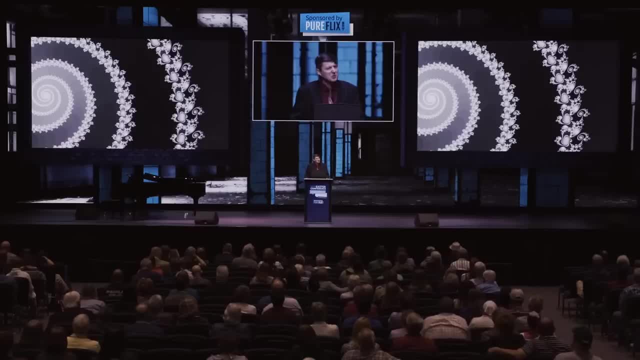 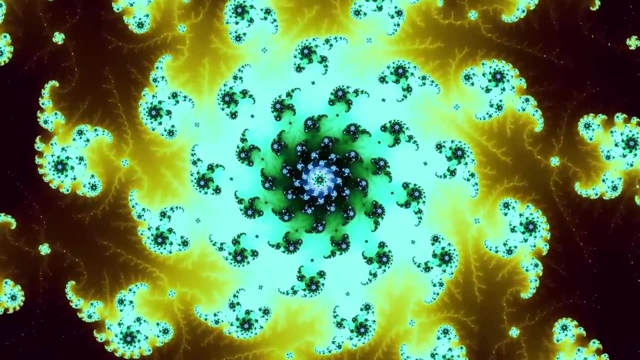 color enhances the beauty of these. even in grayscale they're still beautiful. There's something about that shape that is attractive to us. We see beauty there. I think the color enhances it a little bit. the way putting a little bit of salt on your food brings out the flavor a 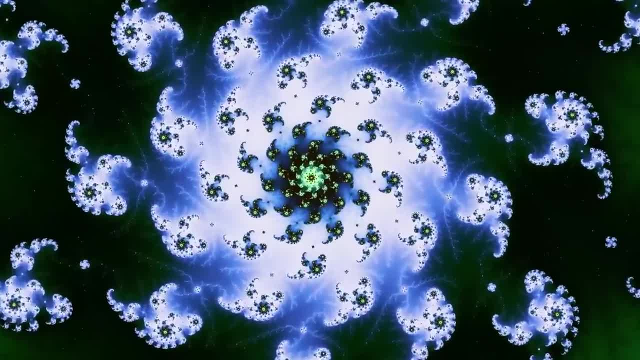 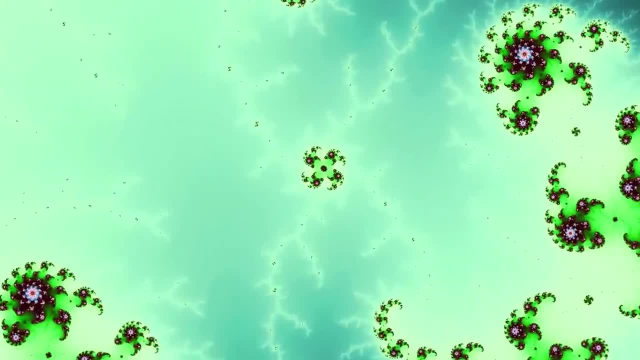 little better, but it certainly doesn't create the beauty. I pick the colors, but the shapes are God's. Is it that the computer create the beauty? Now, you might have said, well, the computer plotted that. but remember, we did the first two points manually. 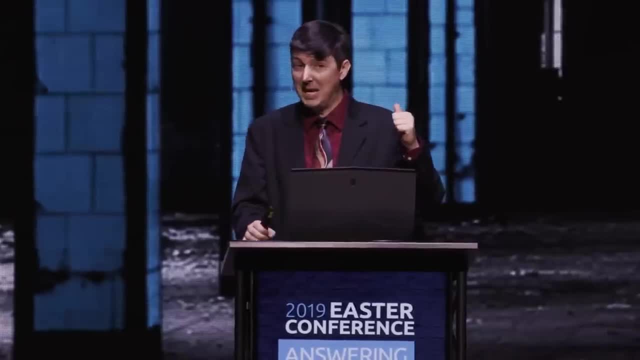 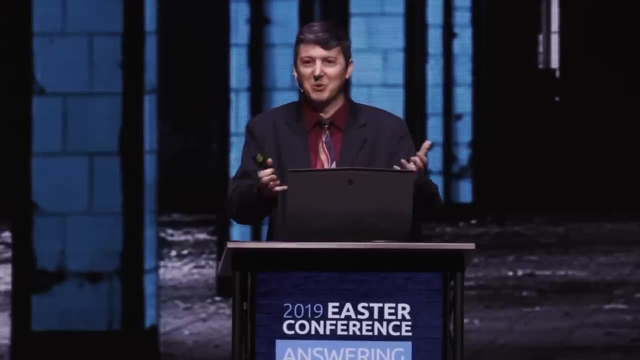 Right, We checked it and ran it through that little form. You could plot this thing manually if you wanted to. It would be horribly tedious, but you could do it and it was. you know. that's why it wasn't until computers that people started plotting this thing. but it's not the computer. 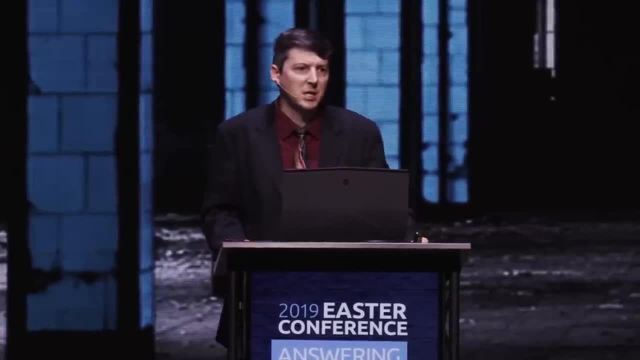 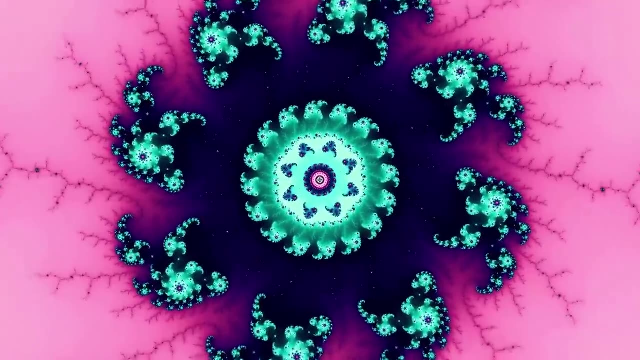 that created the beauty. The computer just revealed it quickly. It did something that would take us a long time to do. It did it fast, but you could do this thing manually. Did people make this? Did Benoit Mandelbrot create the Mandelbrot set? 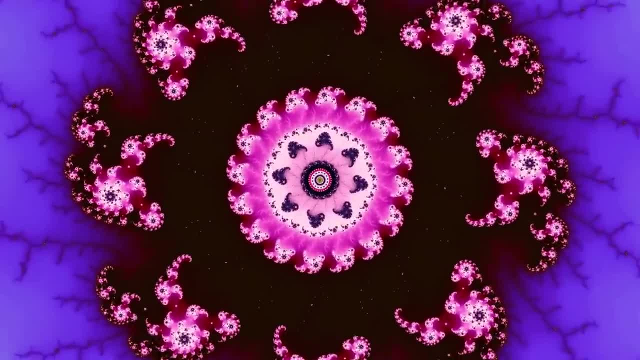 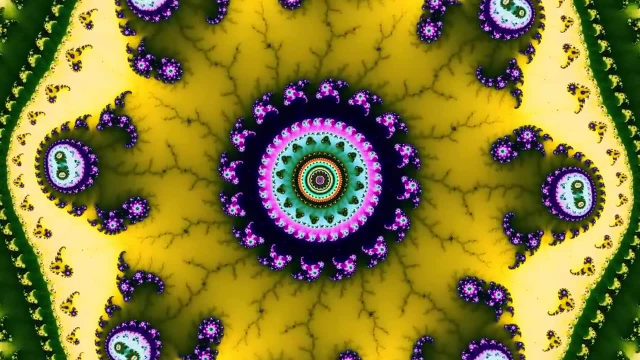 He defined that formula, but did he create the beauty and the complexity? Well, of course not. He was surprised, as was everyone else, and some people didn't believe it. when this was first discovered, They thought maybe it was some kind of artifact, some problem in terms of the way the 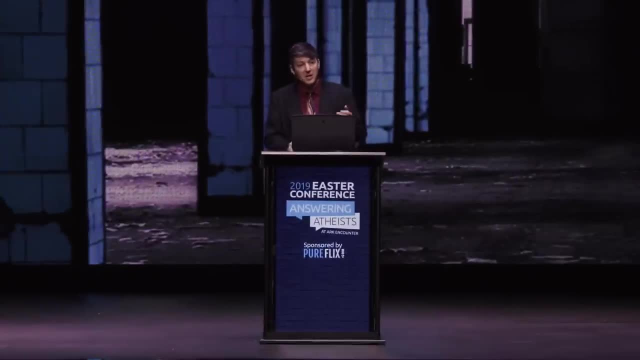 computer is coding, but it's not. That's now been disproved. These things are real. The computer just allows us to view them quickly. People didn't make it. People were surprised by this result. I would say the beauty is built into math. 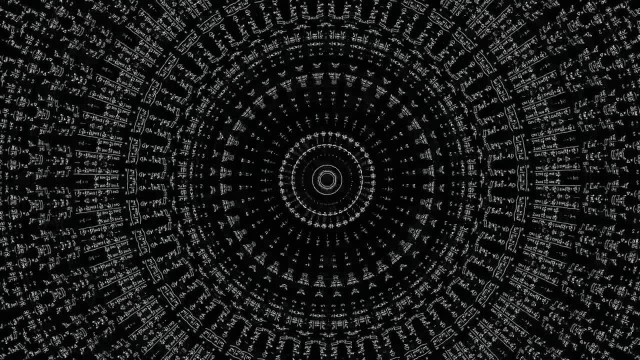 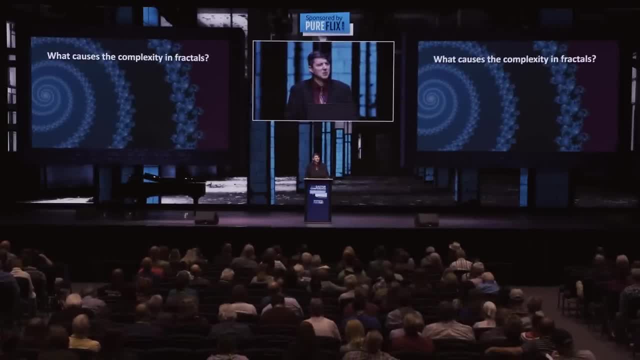 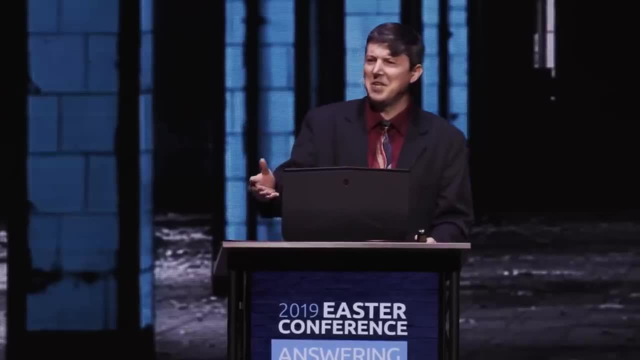 It is. It's always been there, It just has. it wasn't until the 1980s that we had the ability to view it. What causes the complexity in fractals, These intricate shapes that can add and they can and they can count, and so on? What causes all that complexity And the fact that it's 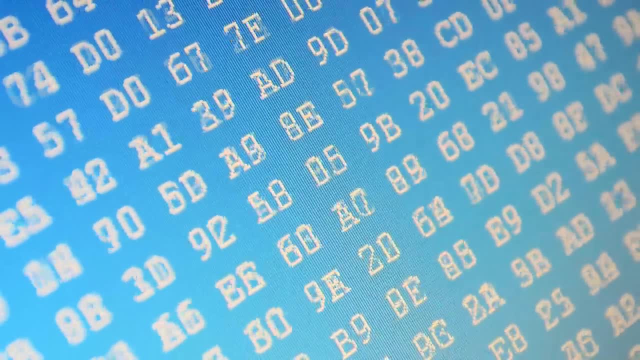 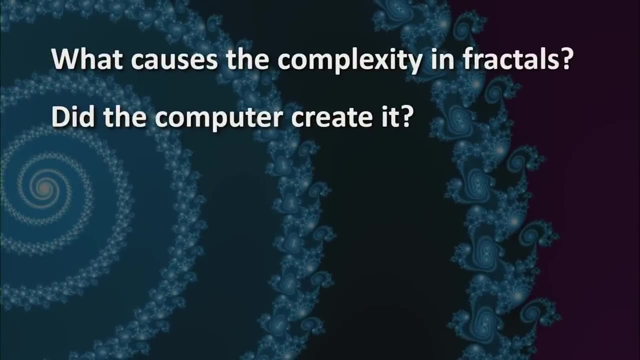 infinitely complex. You have an infinite number of baby versions built in to the original. What's causing that? Was it the computer? Well, again, the computer is simply revealing the complexity. It was already there. The computer didn't create these shapes, any more than a microscope creates bacteria. 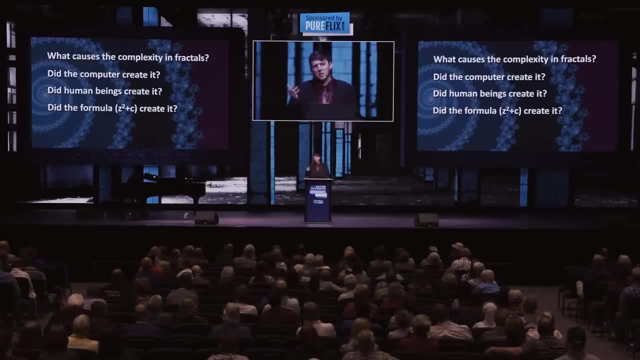 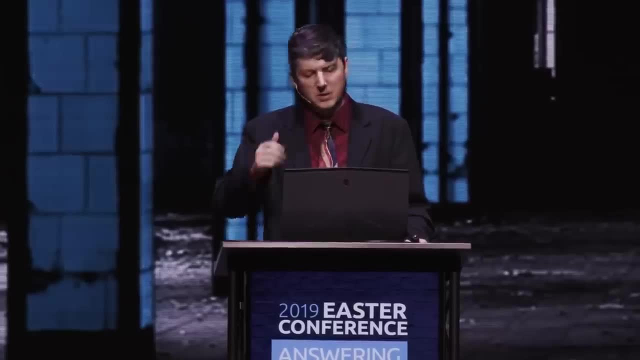 The formula is not that important because you can change the formula. You still get beauty, You still get complexity. In a sense, the complexity is built into math itself. So how do we make sense of that? How do we make sense of beauty and complexity being built into math? What is math? 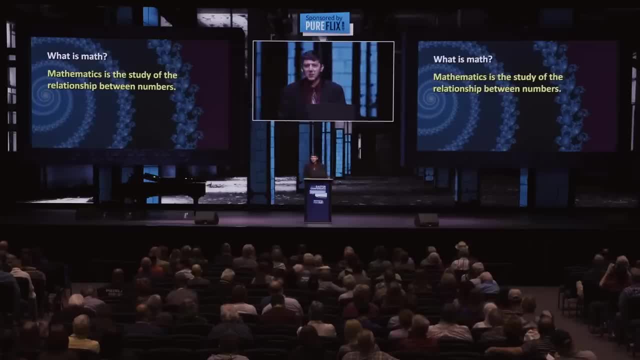 Well, math is the study of the relationship between numbers. right, The rules governing how numbers relate to each other, That's the study of the relationship between numbers. It's pretty easy. And then, of course, I'm going to ask: what are numbers? Well, come on, Lyle, We know. 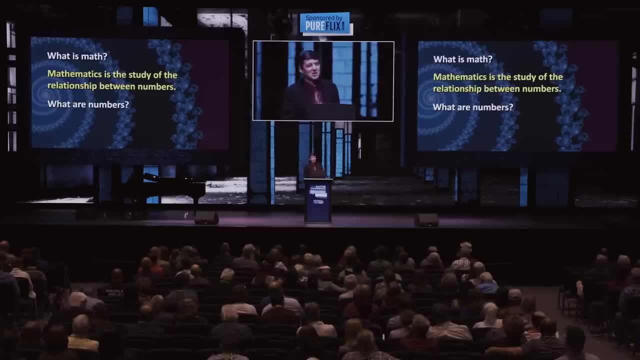 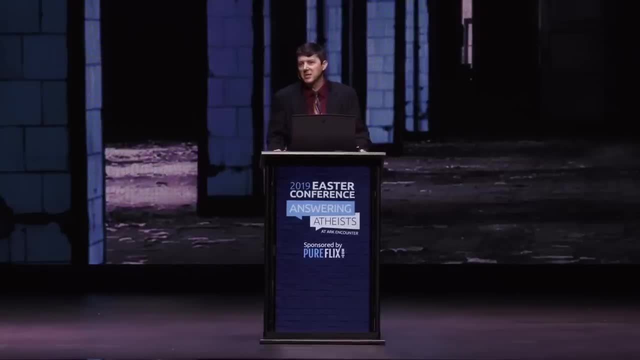 what numbers are. It's funny, Some of these things that are very basic, they're hard to define, aren't they? Like consciousness, it's hard to define it without using another word. that's basically a synonym of consciousness. What are numbers? The best I've been able to find and 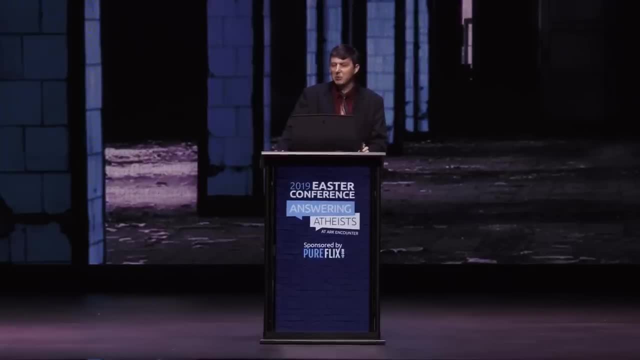 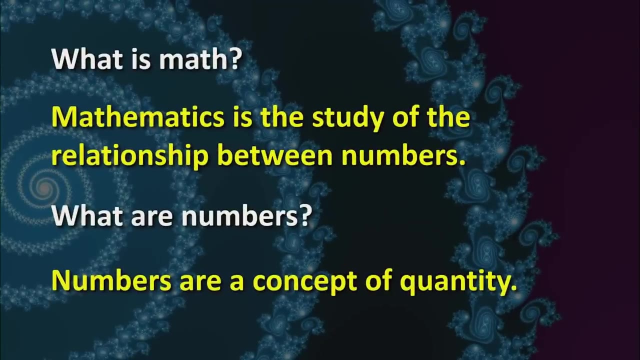 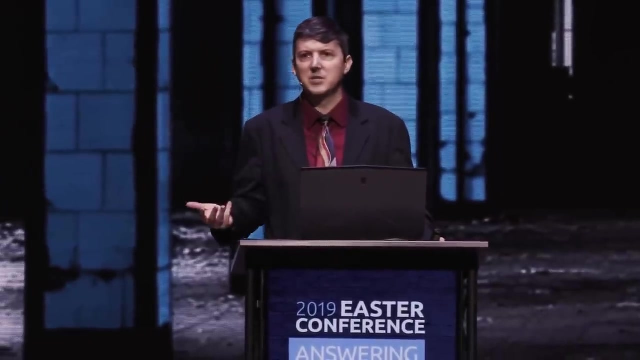 different dictionaries disagree, but the best definition I've been able to find is that numbers are a concept of quantity, And I think that's a pretty good definition. That's the best I've seen. Numbers are a concept of quantity. So if you have three apples, the apples are physical, right, But the threeness is a concept. 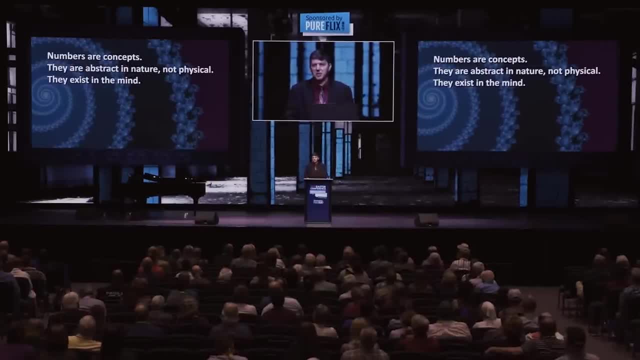 It exists in your mind. You can't physically touch a number, You can't literally see a number. by the way, You might say: well, wait a minute, I see the number three there. Is that really the number three? If it is, then I just destroyed the number three. 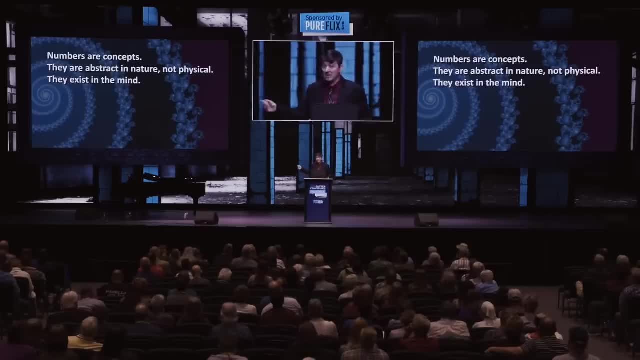 and students. poor students will not have to count one, two, four and so on, because you said that was three and I removed it, so there's no more three. Well, obviously that's not the number three. That's a representation of the number three. right? It's a written numeral. Numerals are not. 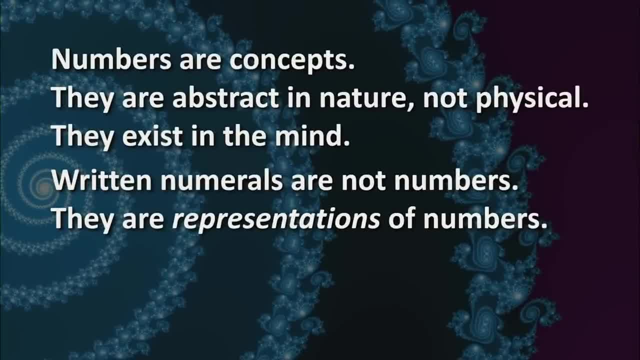 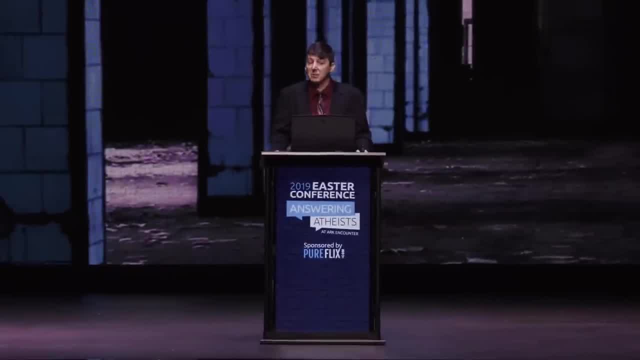 numbers. They're representation of numbers, And we, you know, at some point in history, we decided that shape would represent three things. And, of course, you know, you can use Roman numerals if you like, and they have a different notation. They represent the same concept though, don't they? 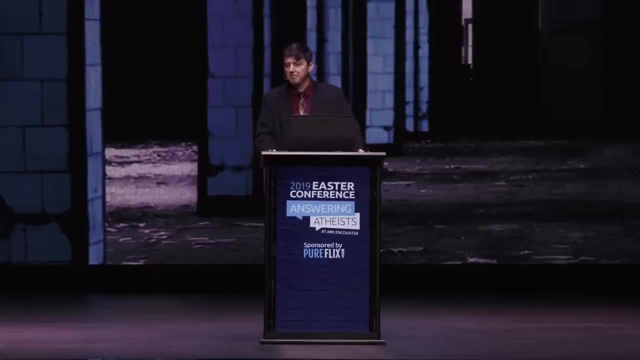 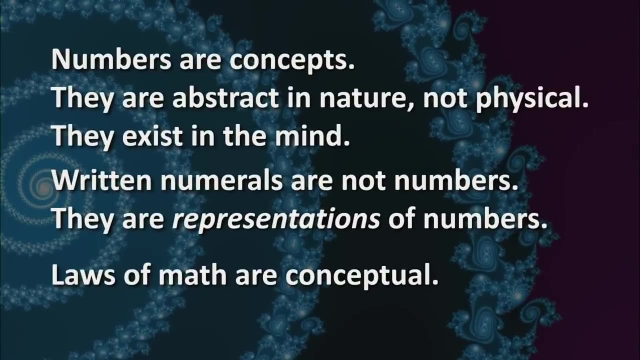 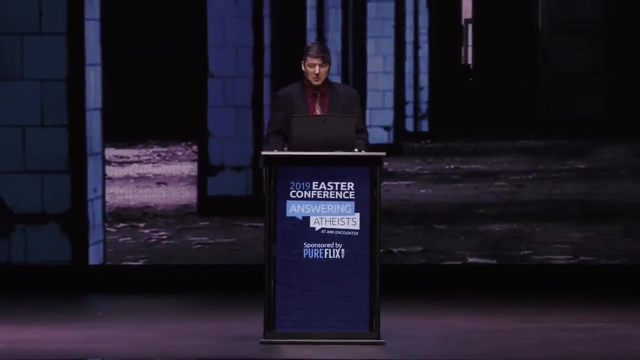 So the concept. that's not something we created. Laws of mathematics are conceptual, not physical. You can't stub your toe on a law of mathematics. You can't stub your toe on a law of a number. You can stub your toe on something that's physical, but not on numbers, because 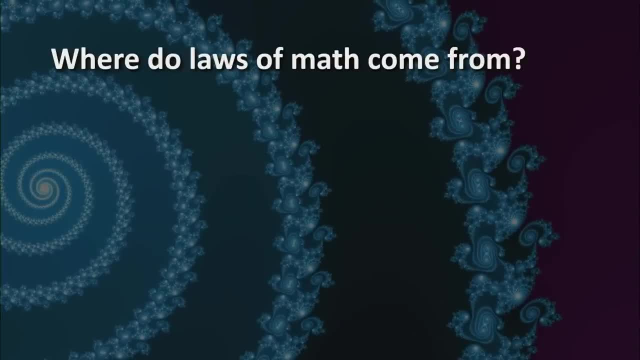 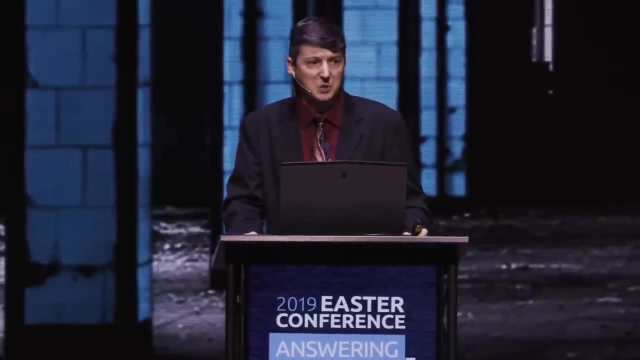 they're conceptual. So where do laws of math come from? This is the question that gets back to origins, right? Because the secularists try to explain everything naturally, and especially by evolutionary processes. So, but did laws of math evolve? That's something to think about, I mean. 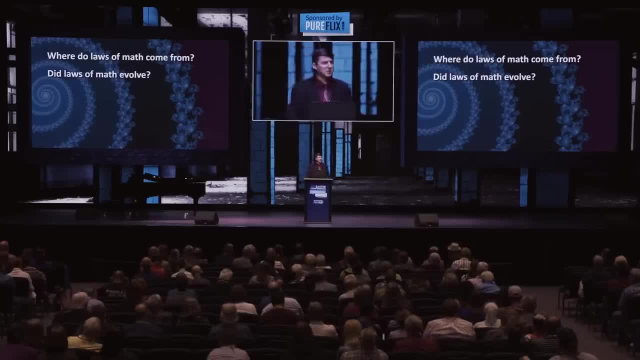 we find lots of patterns in nature. We find, you know, different patterns in animals and the way animals are classified and the way…. Secularists explain that is evolution. They say, well, they had a common ancestor. and then they: 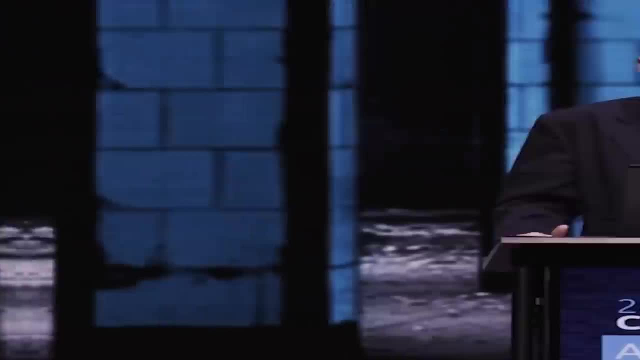 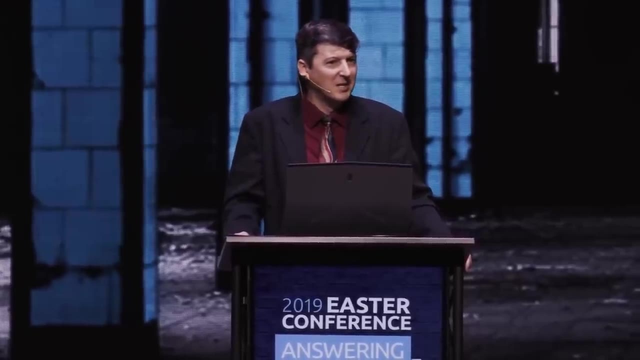 evolved, they changed. Will that work? for math? Did seven used to be three, but it evolved. That doesn't make any sense, does it? Numbers are what they are and they've always been what they are. Laws of math didn't evolve. It's not. like you know, the Pythagorean theorem wasn't true. 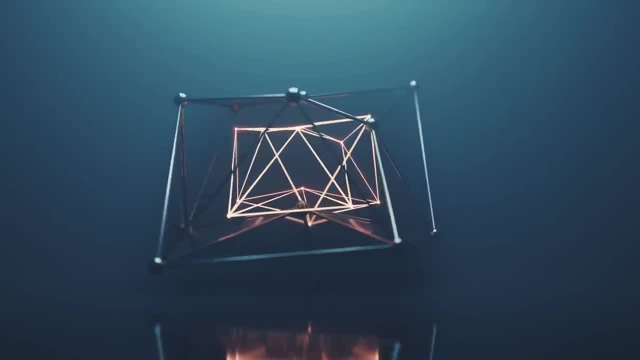 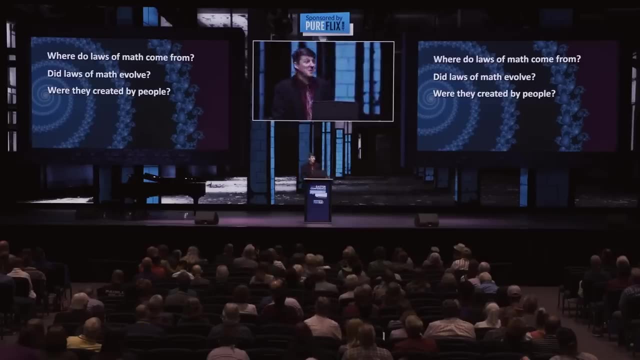 but then eventually, you know, triangles came. No, no, they don't evolve. Laws of math have always been the way they are. Hmm, Were laws of math created by people? Some people argue that, but that's a ridiculous assertion, because if we created them, we could. 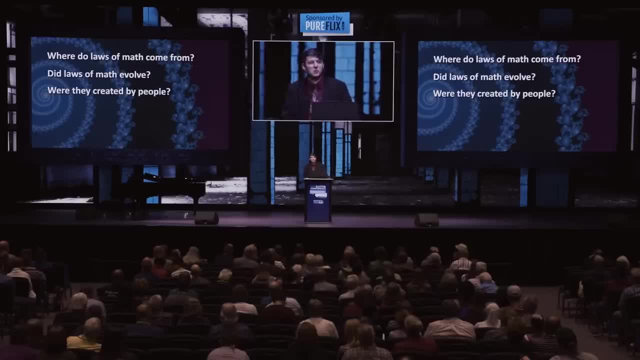 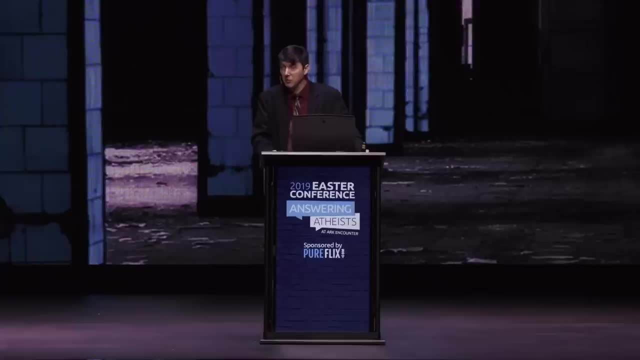 have created them different. We could have said: you know what? Let's all agree that two plus two equals five. Now you could imagine an architect trying to live out that philosophy. It's not going to work out well for him. or try that at your bank. That's not going to work because it just 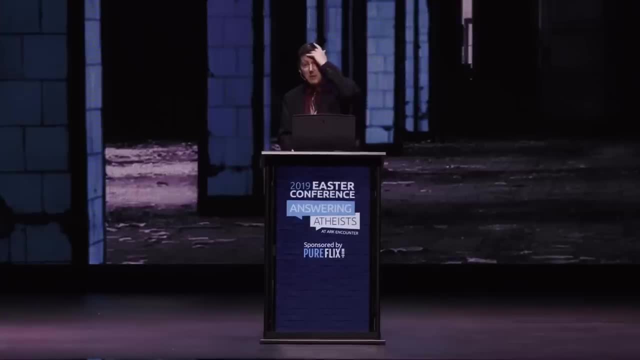 does…. it's not true to reality. We did not create laws of math, We discovered them. Pythagoras, right, He wasn't the first, He wasn't the first to discover, but the Pythagorean theorem right Now. did triangles not add up that way before Pythagoras? 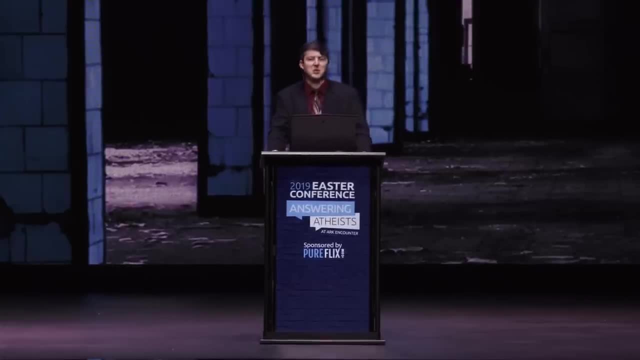 Well, of course they did. He just discovered it. The planets, the way the planets orbit. they obey mathematical laws, Kepler's laws: P squared equals A cubed in terms of the relationship. Was that not true? before people came along, Planets orbited perfectly well for the two days before. 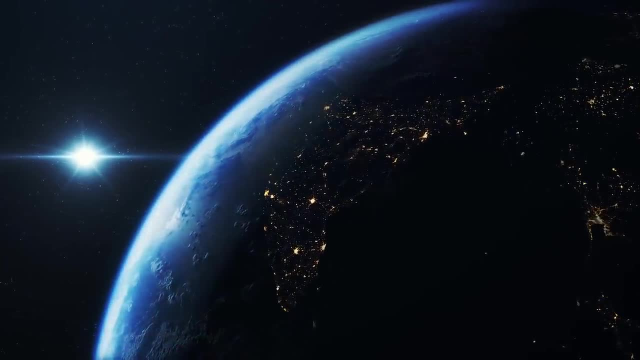 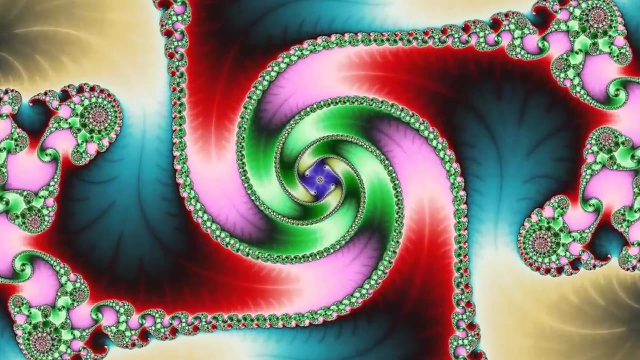 people Now. fractals, perfect fractals, the kind we've looked at so far, repeat infinitely. You can zoom in on the Mandelbrot set forever and you will continually find smaller and smaller versions, baby versions of it. You can do that forever or until your computer blows up. 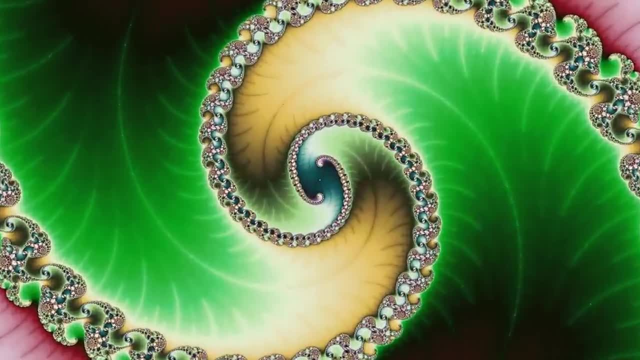 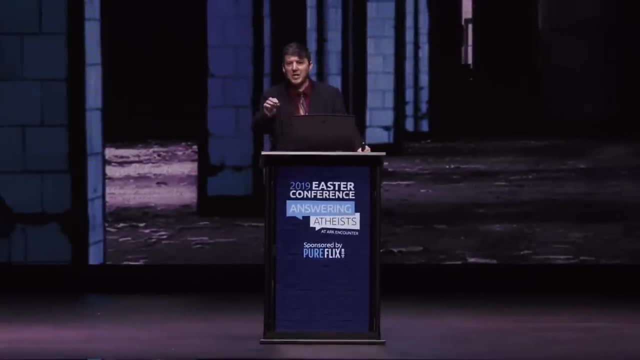 So perfect. fractals repeat infinitely and are only found in the conceptual world of mathematics. Nonetheless, the physical world contains proximate fractals, things that… they go so many steps and then eventually they break down into atoms, and atoms are not fractal. 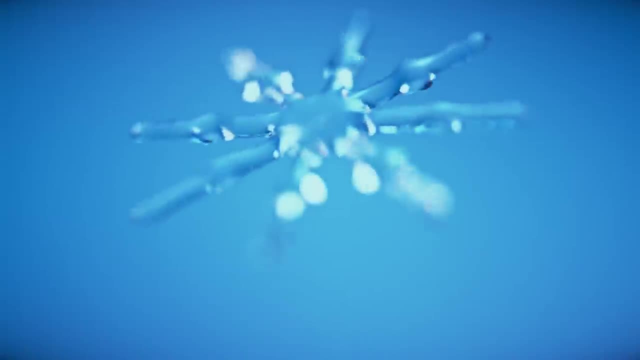 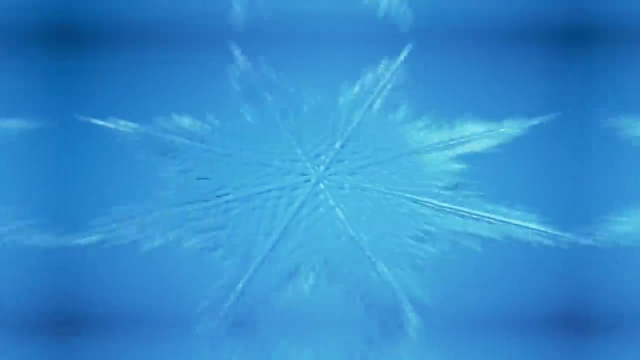 But let me give you some examples of these Snowflakes. Snowflakes have a… fractal quality to them. They have that six-fold symmetry. You zoom in, you still get six-fold symmetry. You zoom in, you get six-fold symmetry. These little gems that God sends us from heaven. 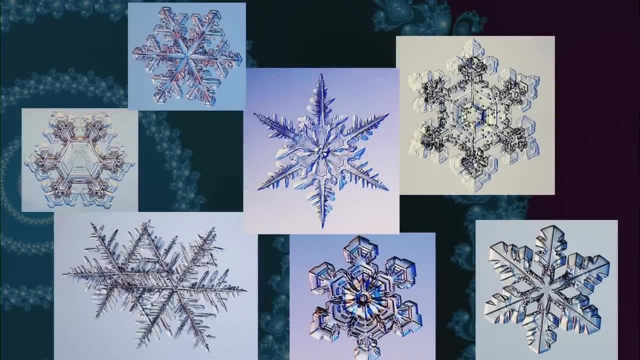 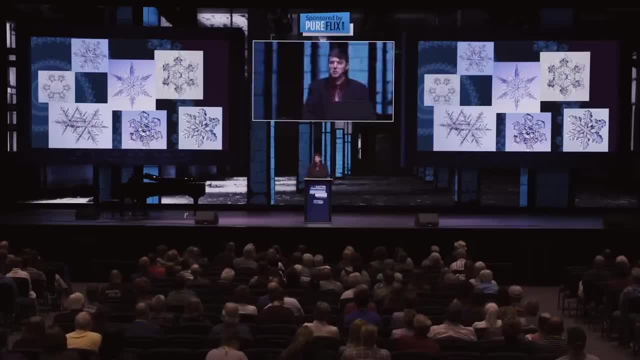 every year and you brush them off the car and, yeah, they're beautiful and they're fractal. They don't repeat exactly, but nonetheless the six-fold symmetry continues no matter how much you zoom in, And so it's hard to tell the size of a snowflake unless you have something to compare. 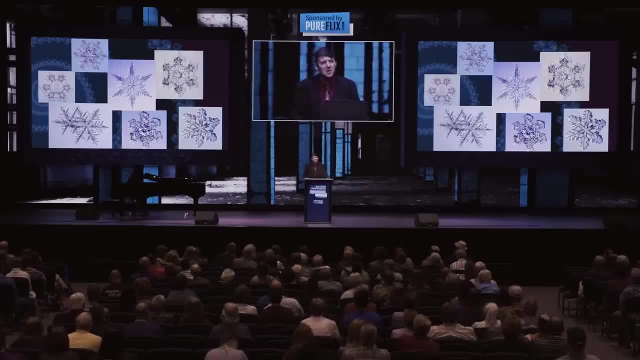 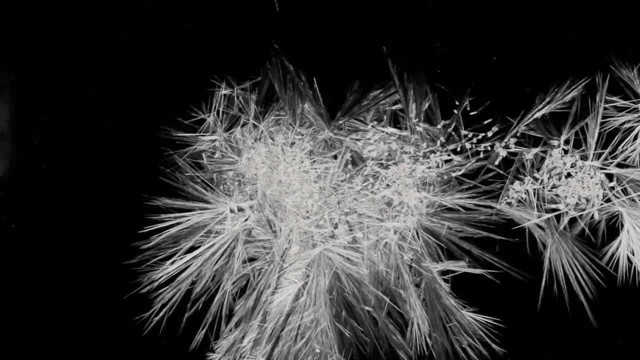 it to, because no matter how big it is, it always looks kind of the same. That's a characteristic of fractals, That stuff that grows on your windows in the winter. I was fascinated by this when I was a kid. Really I still am. I think it's beautiful. It grows on your window- Fractal shapes quite. 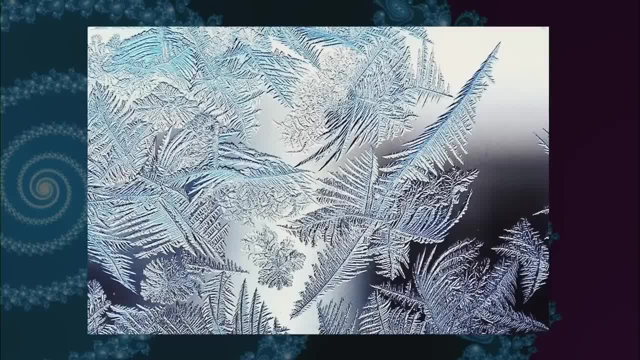 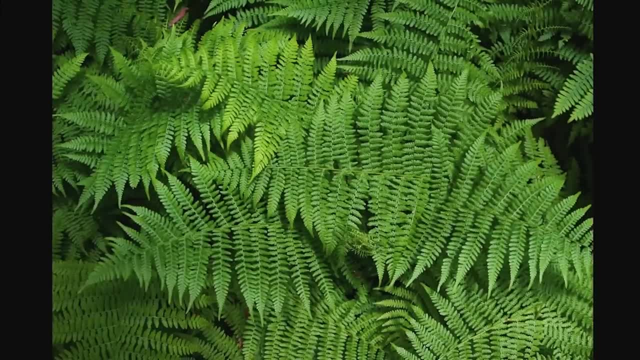 lovely in terms of the way they repeat, They branch and they branch into branches and so on. Ferns are fractal because you see, ferns have a stem and they have another stem growing off of that, and another stem growing off of that and the little leaflets and so on. They branch. 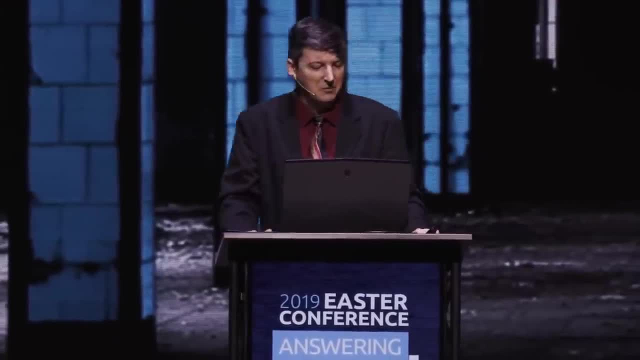 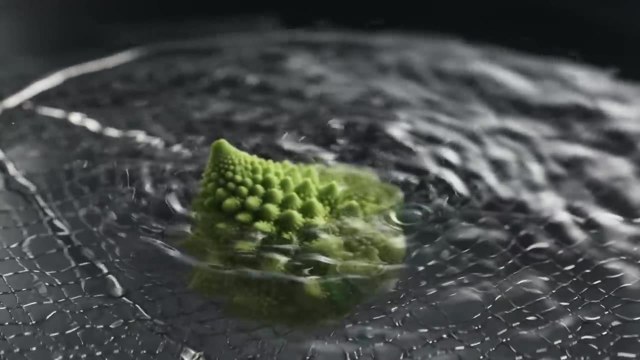 and branch into branches, and branch into branches of branches. I even found a… Fractal broccoli. So I guess broccoli is good for something after all. There you go- Romanesco broccoli- they call that- And you can see it's kind of a cone-shaped, and then it's got cones. 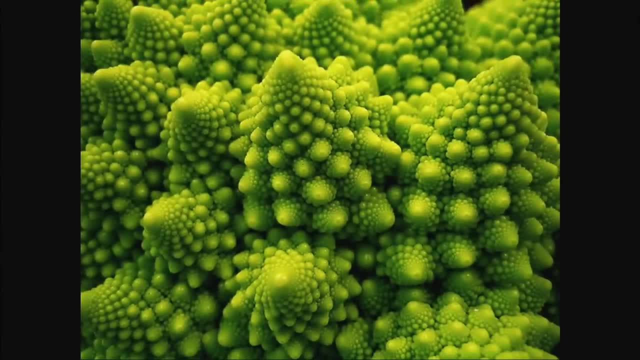 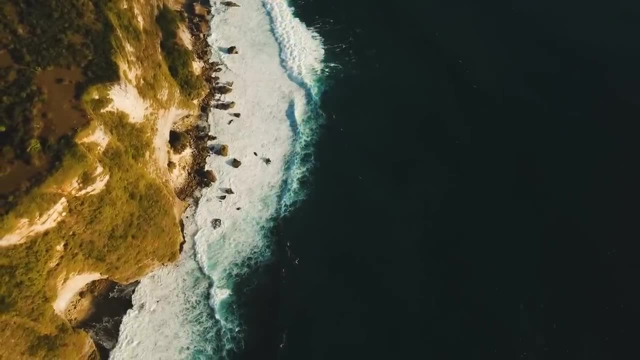 growing on it and cones growing on the cones, on smaller and smaller scales. It's fractal, Isn't that fascinating? Too bad. it tastes horrible. Coastlines are often fractal Coastlines the way they branch. you zoom in on them and they branch into branches and so on. Mountaintops are. 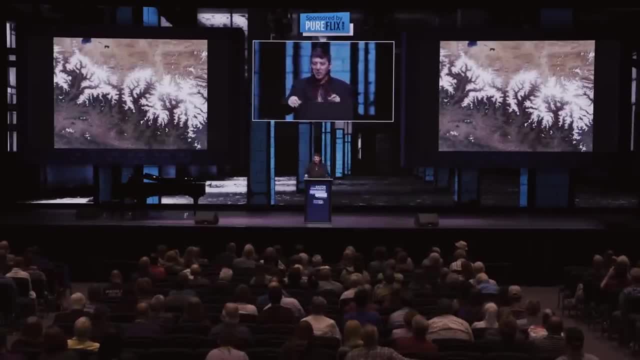 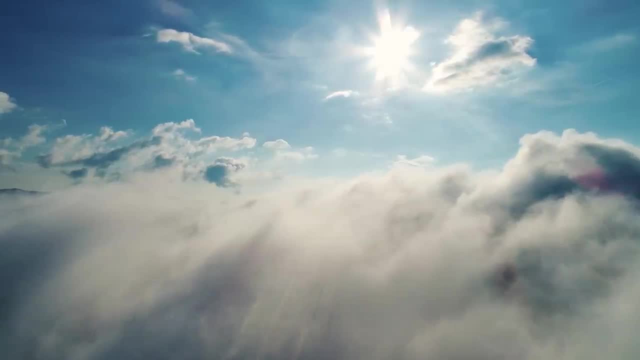 fractal. You look at them from above and they kind of branch and they branch into branches And so on. Clouds tend to be fractal. They don't repeat exactly. but am I looking at the entire sky or am I looking at one very small section of a cloud? It's hard to tell because the same kinds 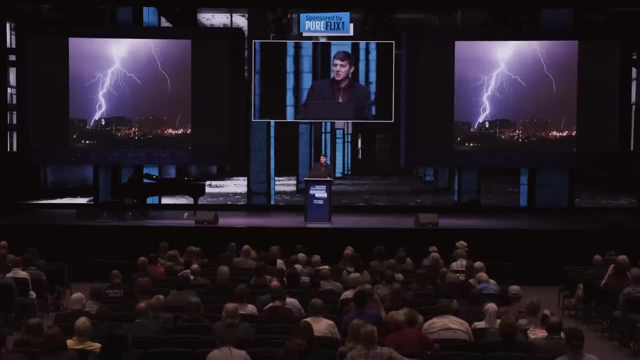 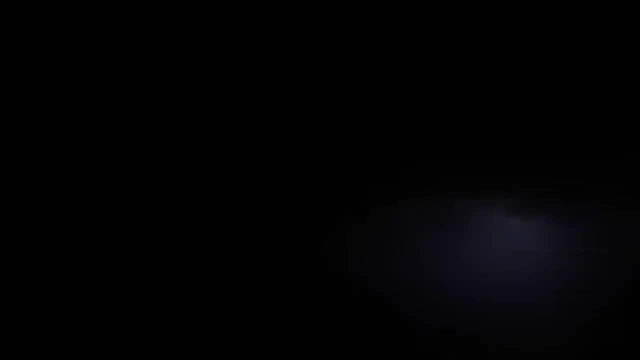 of patterns, repeat The way lightning branches is fractal because you have a main bolt that branches into smaller bolts which branch into smaller ones, and so on, And so lightning very beautiful, and because it has that fractal quality to it And it's really neat too when you 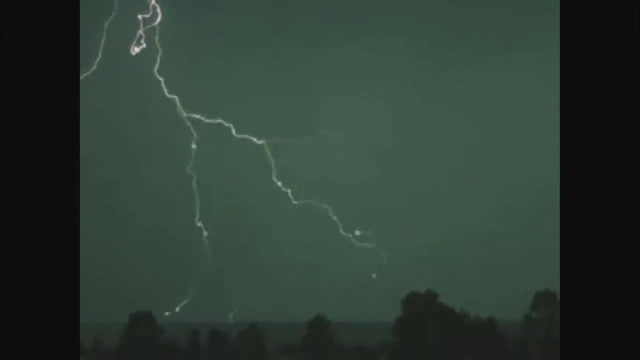 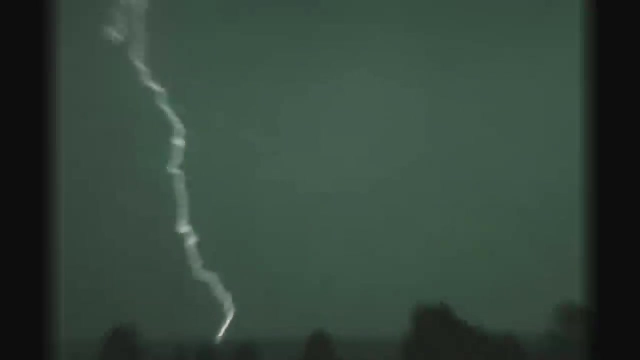 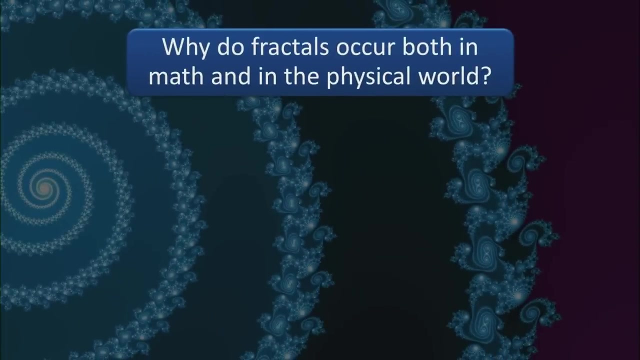 watch it in super slow motion. you can see how it branches out into all these different branches. The leader connects and then most of the current goes down the leader. Quite fascinating. So here's my question then: Why do fractals occur both in math, which exists in the mind? 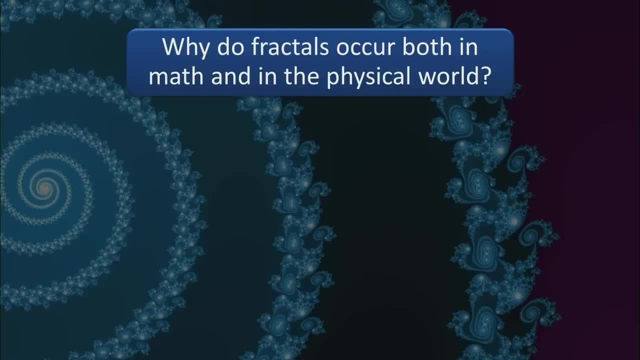 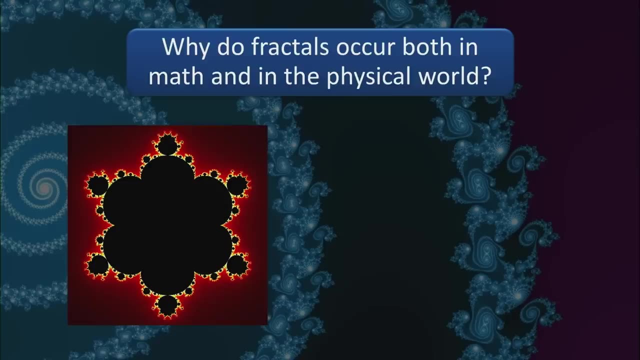 it's conceptual, and in the physical world, which is made up of atoms and does not exist in your mind, Right? I mean, you have this shape that's a multibrot that exists only in the conceptual world of mathematics. We can plot it, but you can never touch that thing because it's not physical. 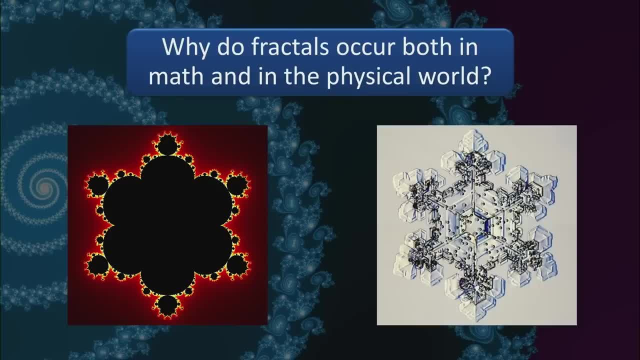 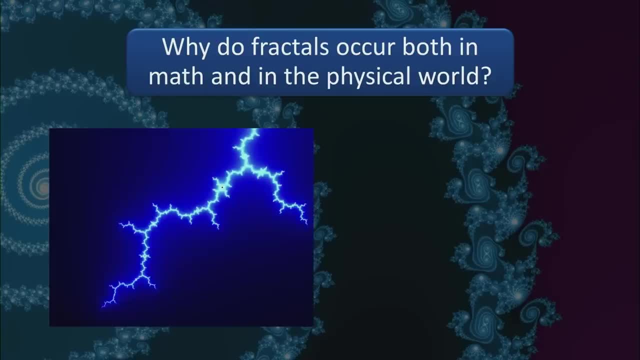 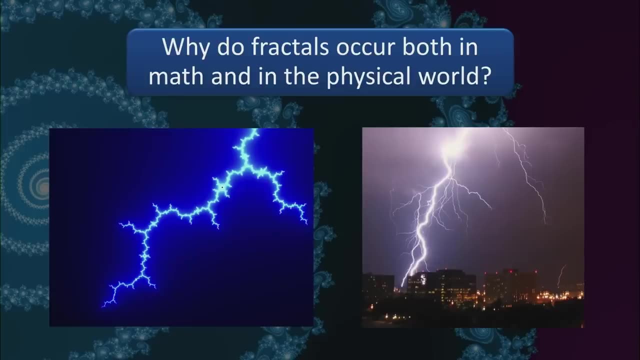 it's not made up of atoms, But that one does, and they look remarkable. They're probably similar. This particular shape here is part of the Mandelbrot set. Looks like a bolt of lightning, but it's not made of atoms. This one is: How is it that conceptual things? 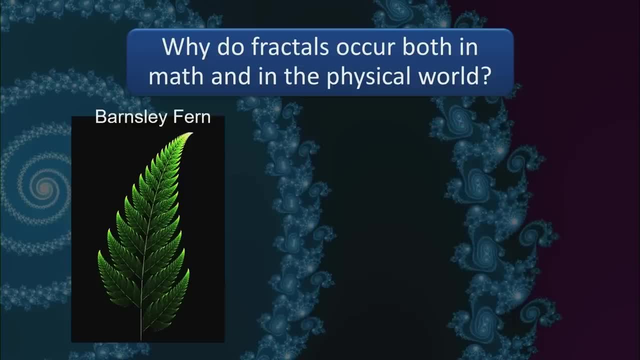 that exist only in the mind also occur in the physical universe. This particular shape that might look like a plant, that's actually a mathematical graph, called a Barnsley fern. And a Barnsley fern is such that each leaflet is the entire shape. Let me show you. 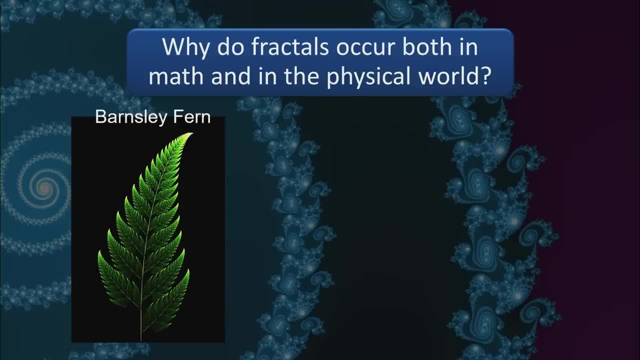 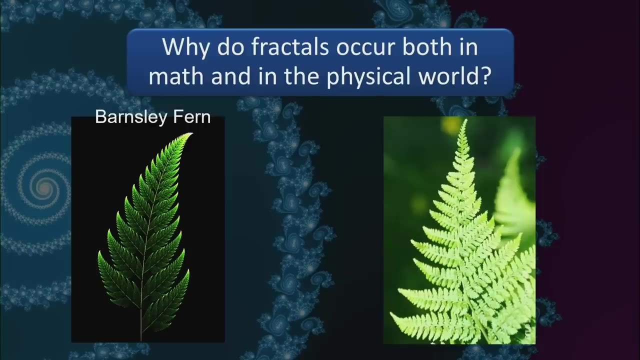 Isn't that interesting. Let's do it again, just because it's cool. See the entire shape. each leaflet is the entire shape- Fascinating. You can't touch that, though It doesn't exist in the physical world, but that does. That's very similar. This stuff right here. that's a 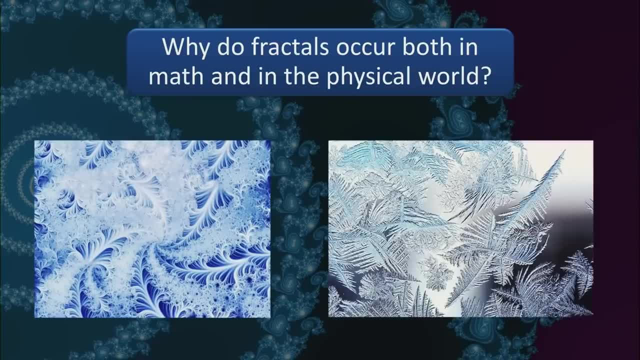 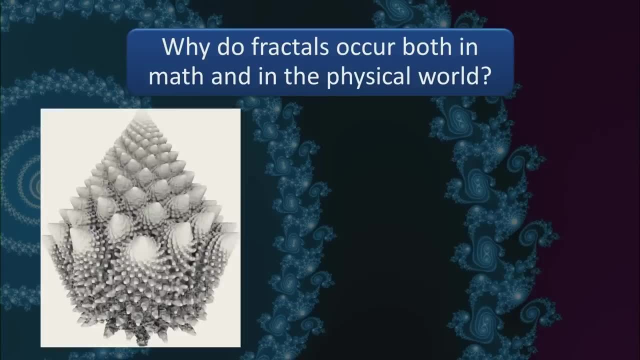 mathematical graph That doesn't exist in the physical world but that grows on your windows. This particular mathematical shape cones on cones. it does not exist in the physical world, Whereas this unfortunately does This particular shape that's part of the Mandelbrot set. 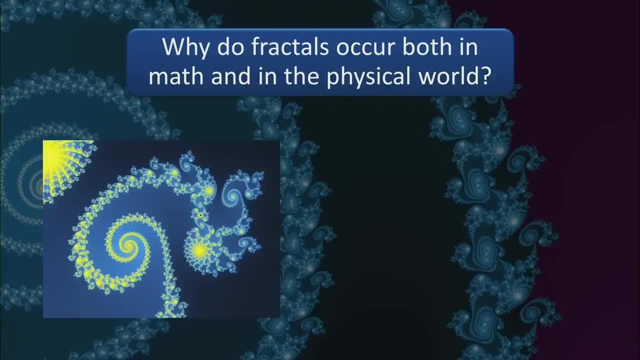 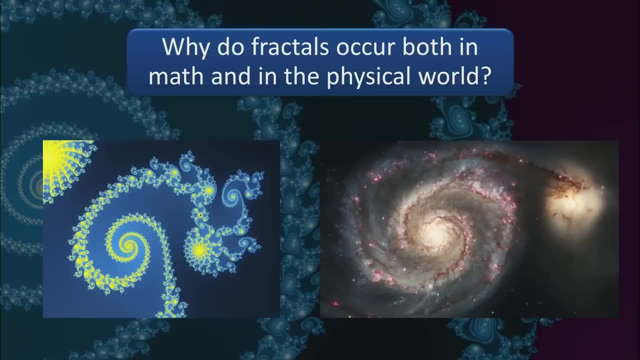 it's a double spiral. You can't see that in a telescope because it's not made of atoms. It doesn't exist physically in the universe. but that one you can look. you can see in a small telescope The Whirlpool Galaxy not too far off from the Big Dipper. So how is it that math? 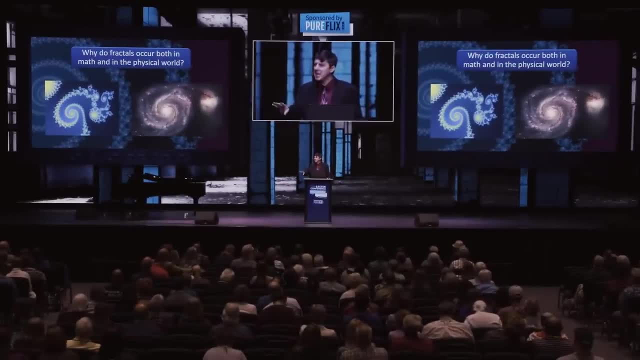 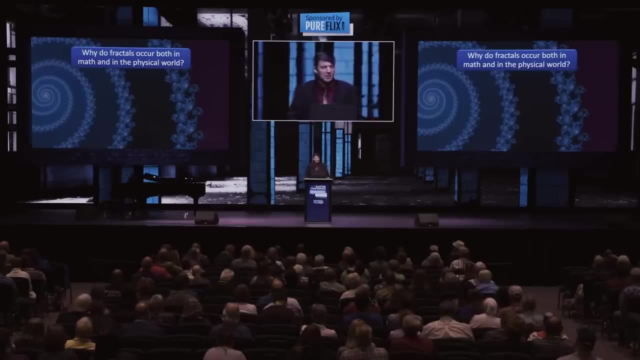 which is conceptual, you find these shapes, and then in nature, which is physical, you find the mathematical laws. Now, one answer to this- and a skeptic might say this is: well, the physical universe obeys mathematical laws. So it stands to reason. if something can occur in math, it can. 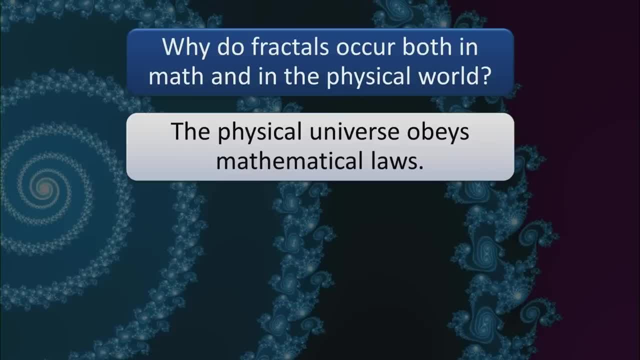 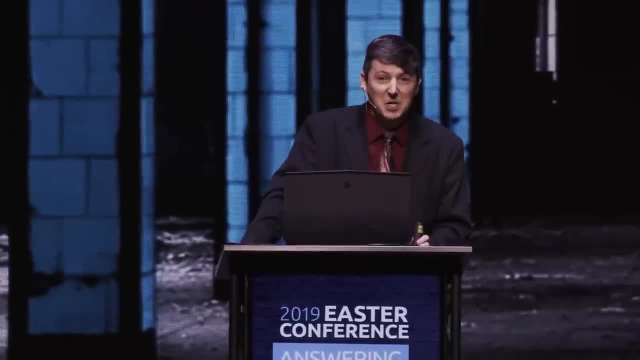 occur in the physical world because the physical world obeys math. Okay, I'll grant that. But then I'm going to have to ask: why does the physical universe obey mathematical laws? And that is a stumper. if you're not a Christian, If you're not a Christian In the Christian worldview, I can make. 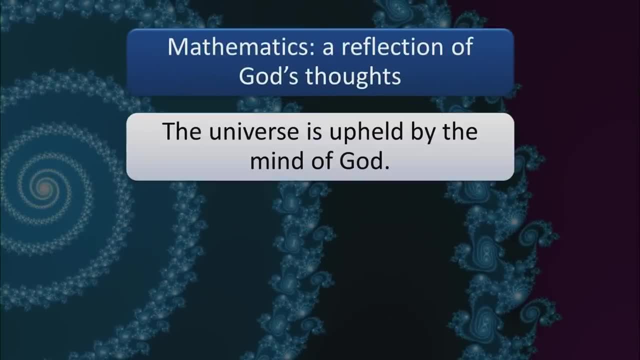 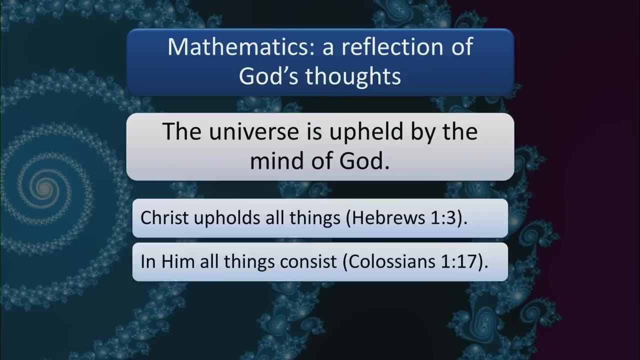 sense of why the physical universe obeys math. Because the universe, the physical universe, is upheld by the mind of God and God thinks mathematically. So it stands to reason. the physical universe will obey mathematical laws because God upholds all things by the word of His power. the Bible says: and in Him all things. 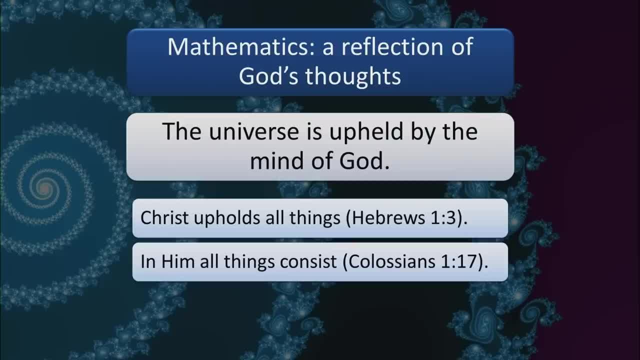 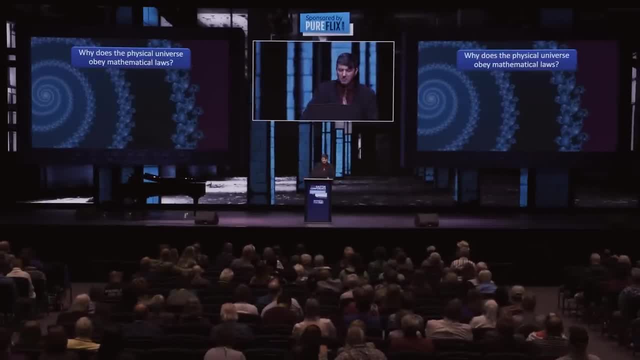 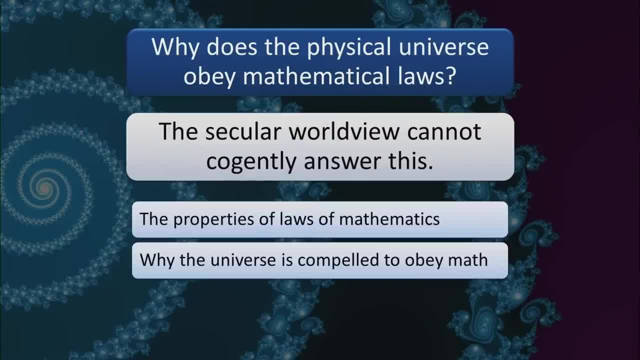 explain it. They can't explain it. They can't explain the properties of laws of mathematics, why they are conceptual, universal, abstract, invariant, exceptionless, and why the physical universe is compelled to obey them. Why would a physical universe obey conceptual laws You come up with? 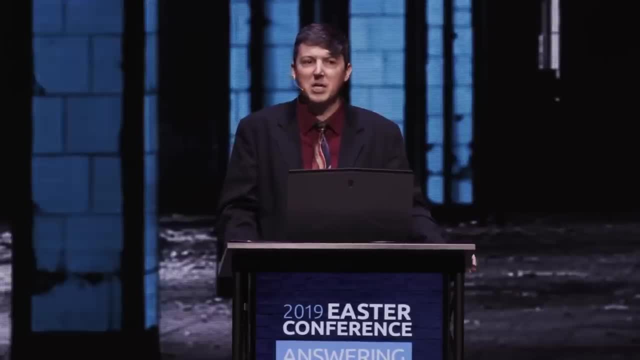 something in your mind, does the universe automatically just obey it? Of course not. It doesn't make sense, Unless you think I'm making this up. some brilliant people have written on this topic: Dr Eugene Wigner, who is a PhD physicist. I believe he's a Nobel Prize winner. Brilliant man. 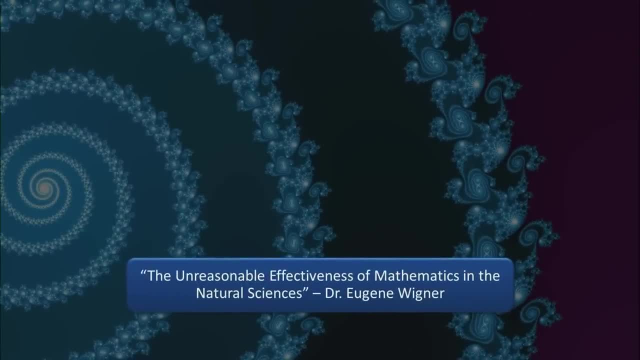 He wrote a wonderful article years ago. I love this article called The Unreasonable Effectiveness of Mathematics and the Natural Sciences Interesting. Now he's coming at it from a secular perspective and from a secular perspective, he's perplexed. It's unreasonable. 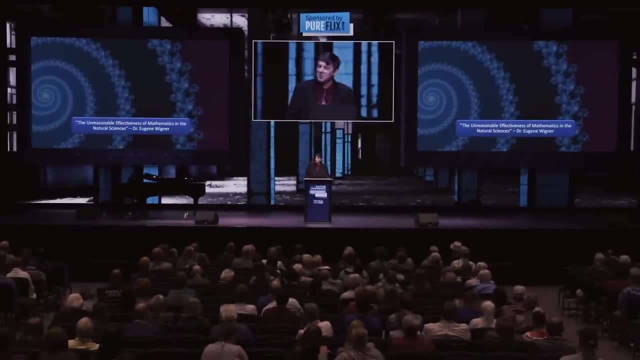 that mathematics should work so wonderfully in explaining the physical universe, mathematics being abstract the universe, the physical universe being physical, And so he discusses this in the paper. this perplexing dilemma is: why does the universe obey math? He says it's difficult to. 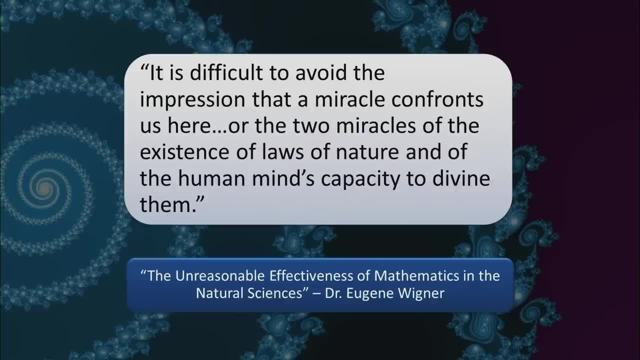 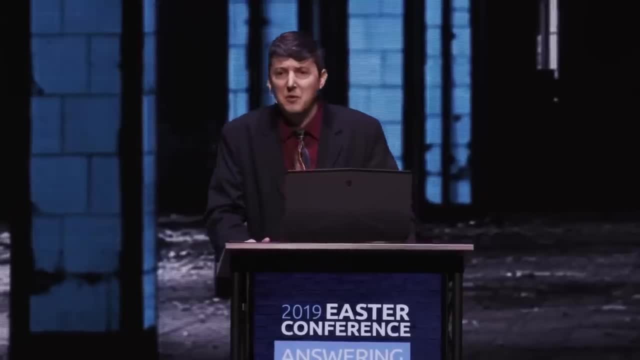 avoid the impression that a miracle confronts us here, or the two miracles of the existence of laws of nature and of the human mind's capacity to define them. He's saying it's amazing, first of all, that the universe obeys mathematical laws. That in itself is astonishing, and what's even? 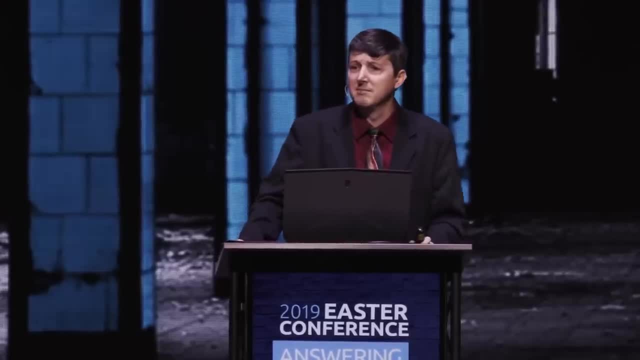 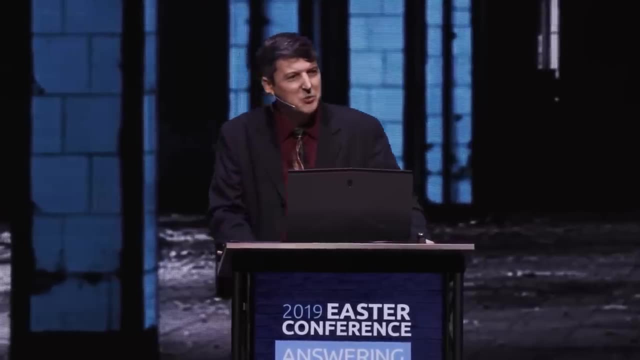 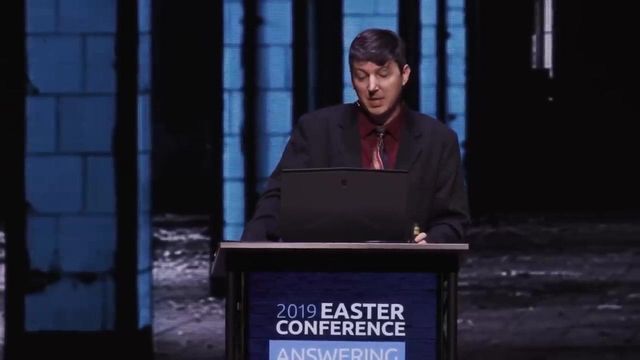 more astonishing is that human beings can discover those laws. That's remarkable, almost like a miracle. Yeah, What is his conclusion? Does he come up with an answer from a secular perspective? Here is his conclusion: The miracle of the appropriateness of the language of mathematics for the formulation. 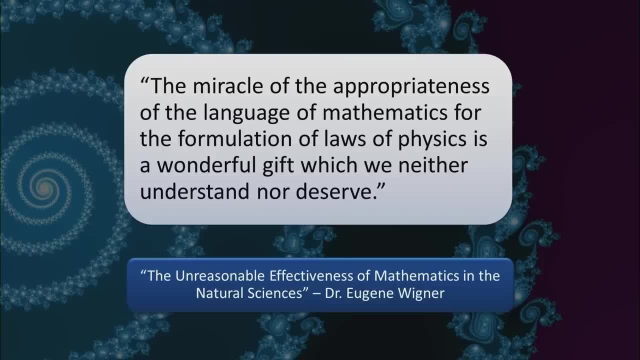 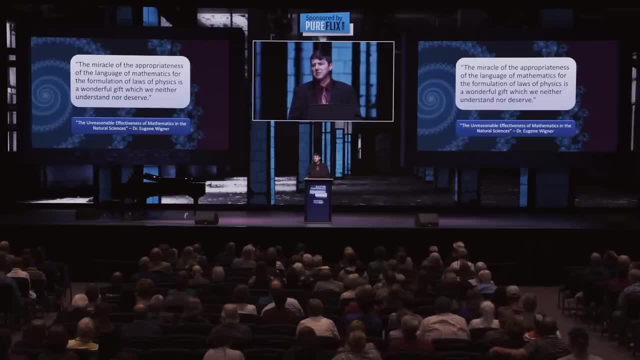 of laws of physics is a wonderful gift which we neither understand nor deserve. Isn't that interesting? There is no answer from the bankrupt evolutionary atheistic camp as to why the physical universe obeys mathematical laws, but it is exactly what the Christian religion is doing. It's not? 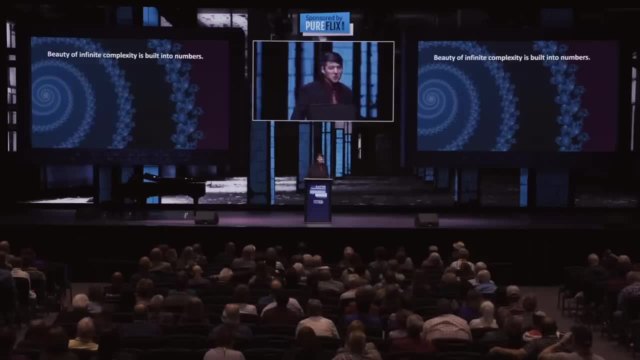 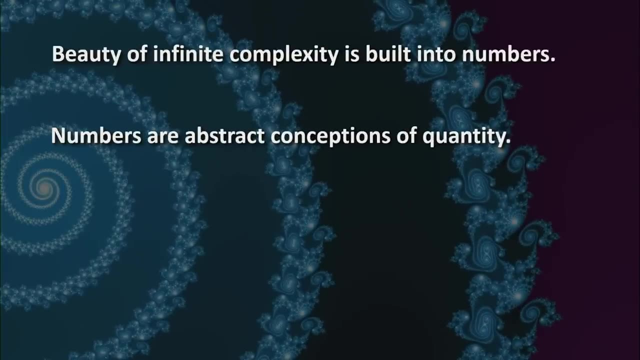 what the Christian would expect. It's exactly what we'd expect. So we've seen that there's beauty of infinite complexity built into numbers. Numbers are abstract conceptions of quantity. They exist in the mind. Concepts require a mind and numbers are a reflection, therefore, of the way God thinks It. 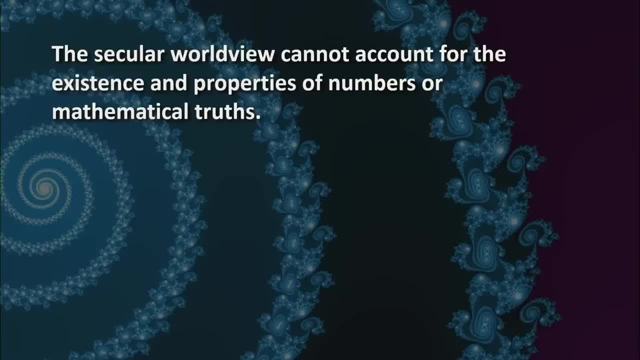 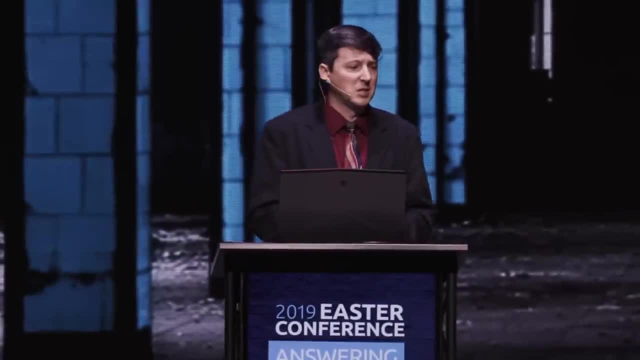 makes sense in the Christian worldview. The secular worldview cannot cogently account for the existence and properties of numbers and mathematical relationships, mathematical truths. It can't make sense of it. It doesn't make sense in their worldview. Numbers existed, but they don't exist. 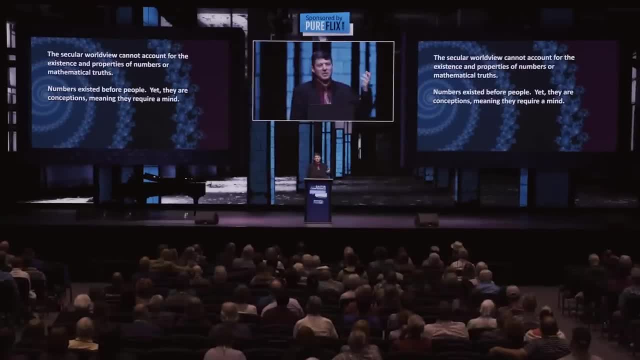 They existed before people. yet they are conceptions, meaning they require a mind, and that means minds existed before people did, And that makes sense in the Christian worldview. We can have that. It makes sense. Laws of mathematics are universal, invariant, abstract entities. It's exactly what.